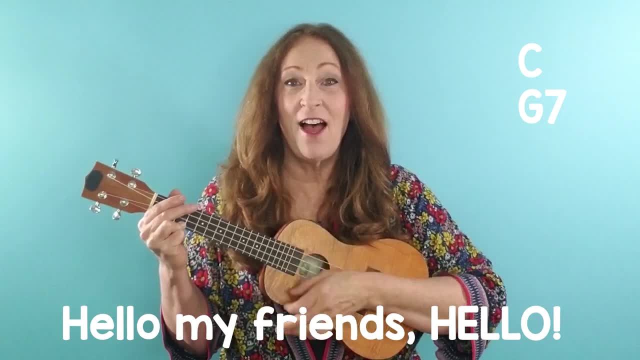 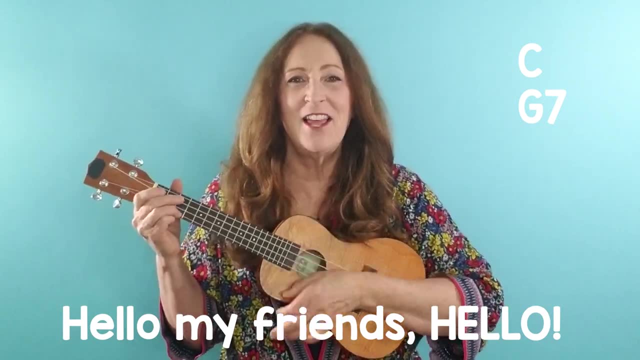 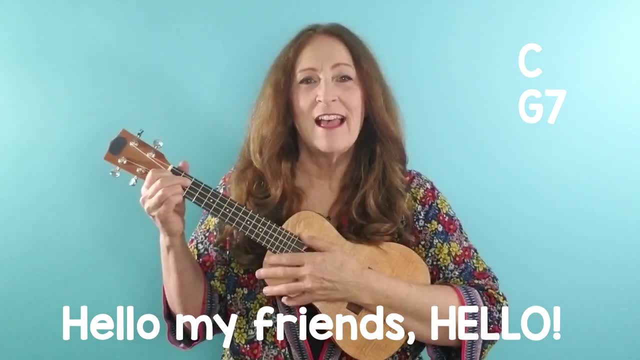 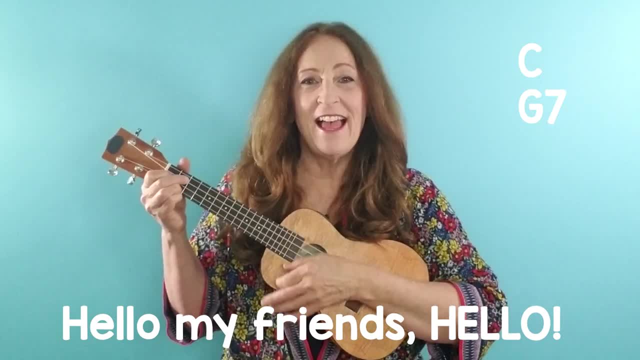 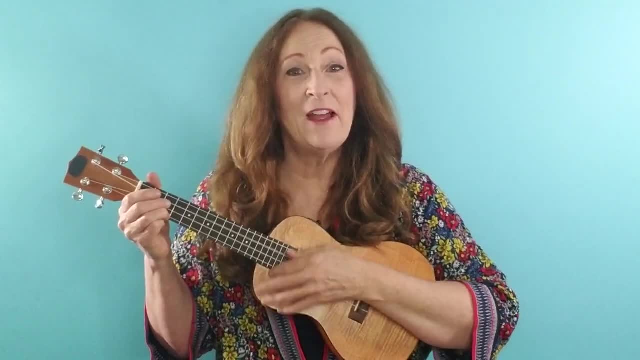 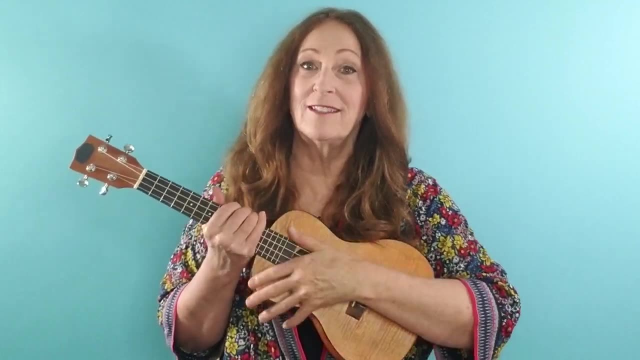 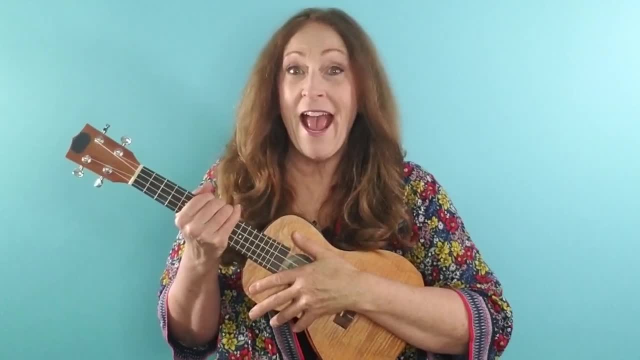 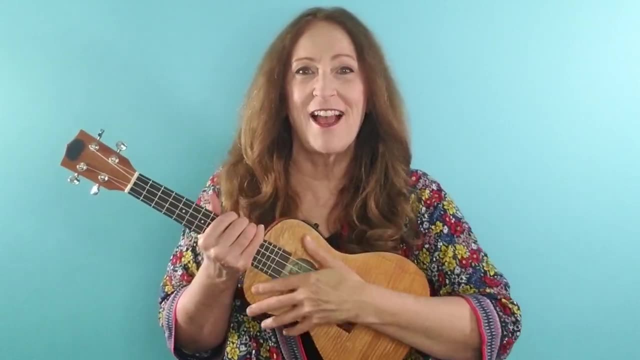 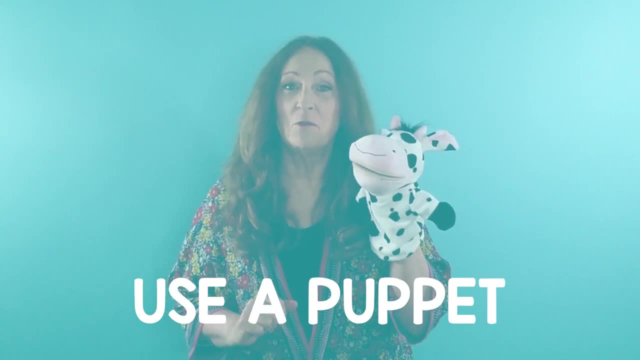 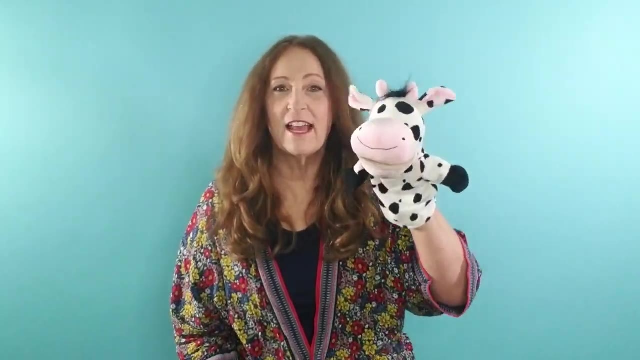 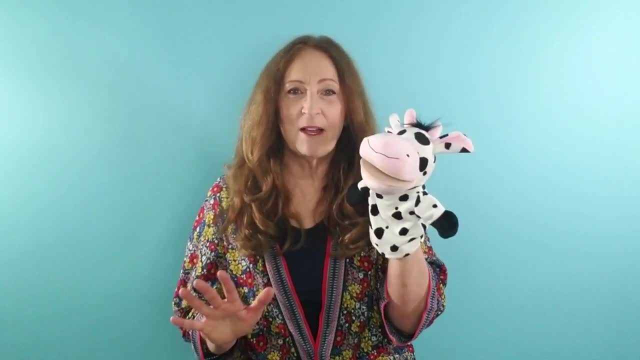 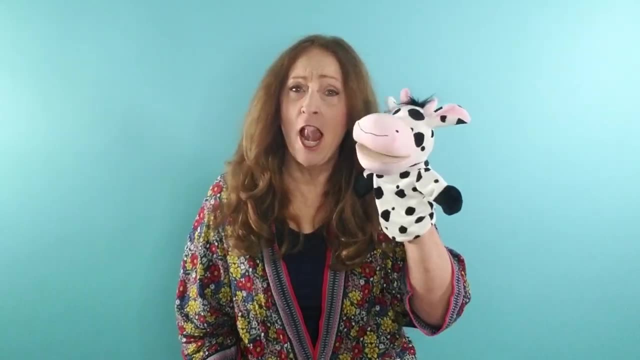 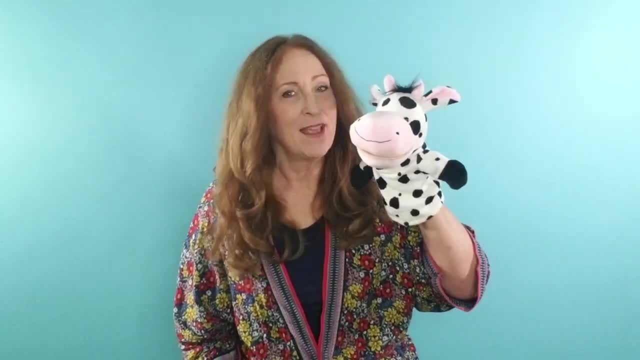 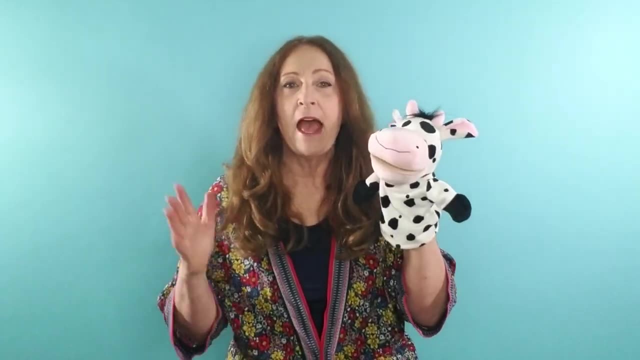 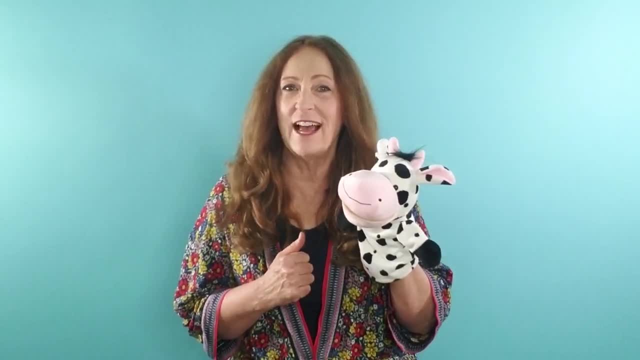 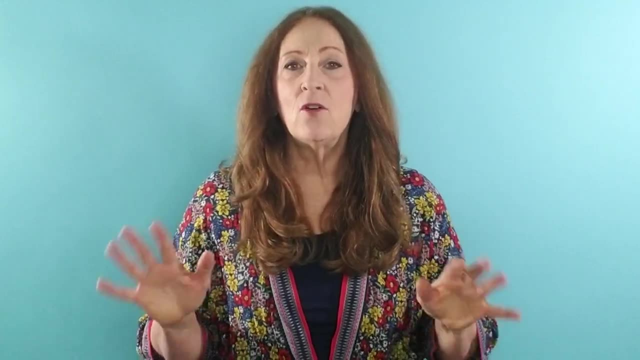 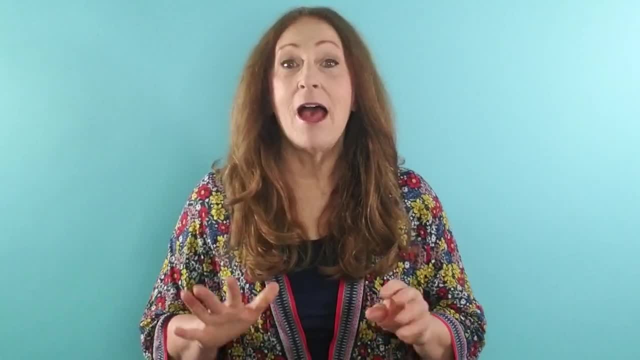 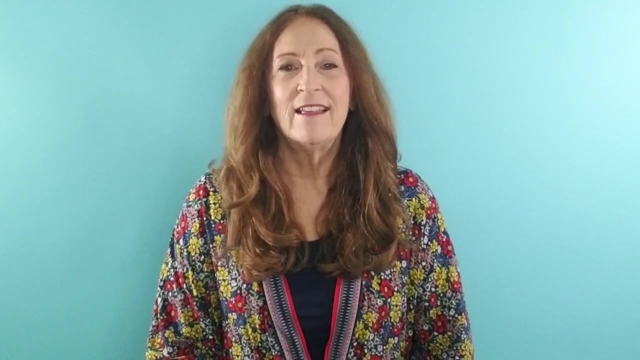 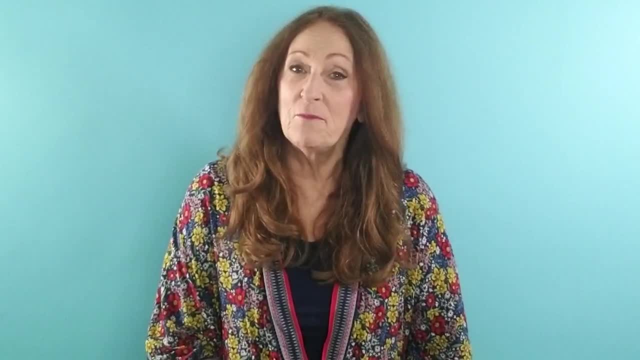 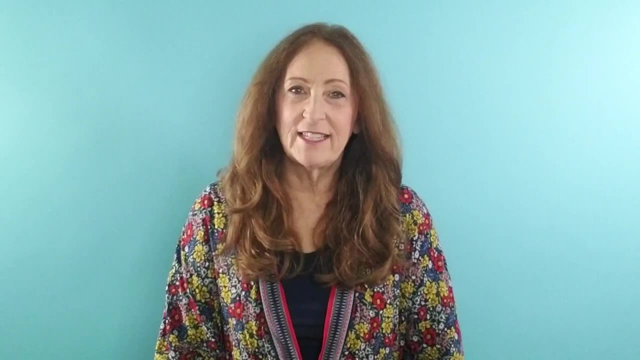 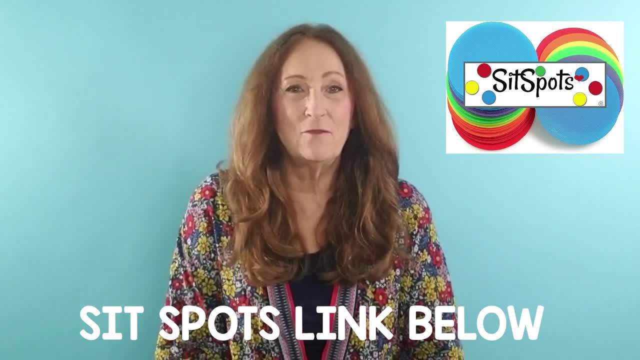 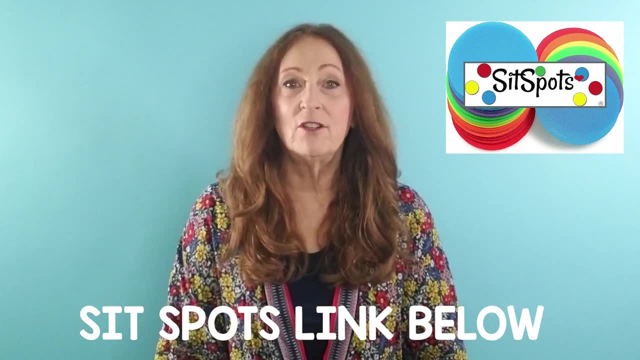 that don't like them. They worked in my classroom. They stuck to the floor, They were stuck on so well, they weren't really a problem. But you can use any kind of marker in your classroom, whatever your seating arrangement is. I know for a bunch of years I was out in a portable and I actually 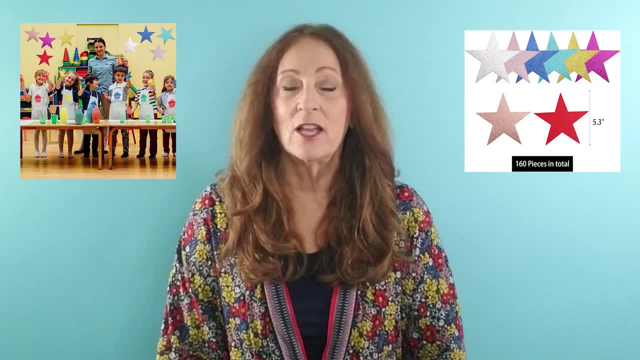 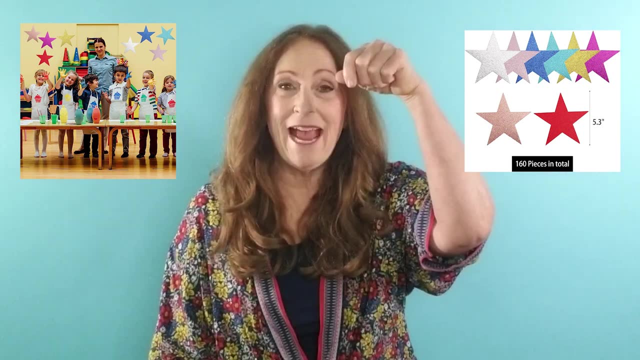 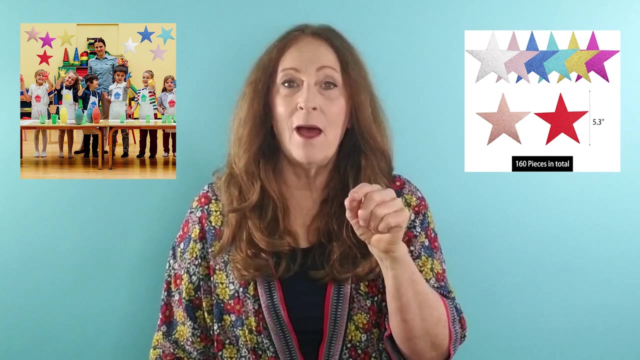 attached some cutouts like stars to the ceiling because it had the tiles and there was a little metal crossbars and I could use a paper clip and hang a clear thread down which was fire safe, and then it had a little star with a number on it And then the kids only had to look up to find. 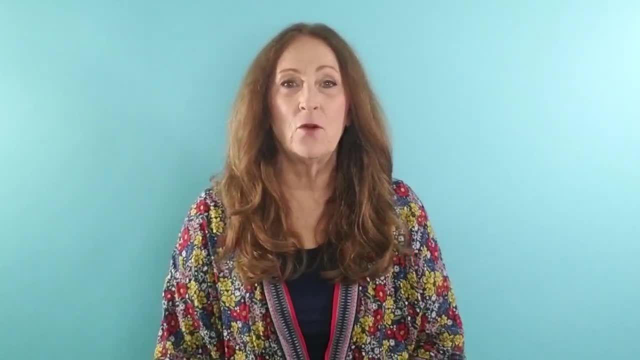 their spot and I didn't have to worry about anything on the floor, and that worked really well too. So it is a good idea to have some way to identify where that set out five while it's unbolted and it's not defects. as a matter of fact, we, DragonX and I- 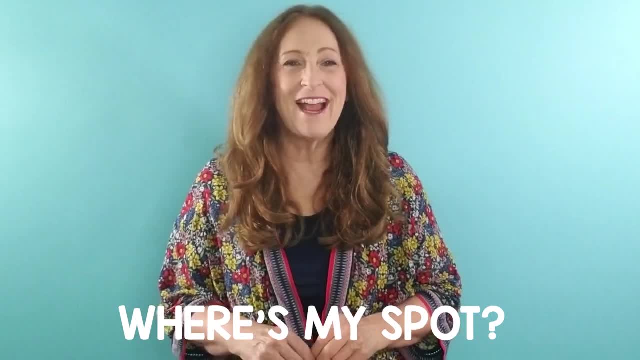 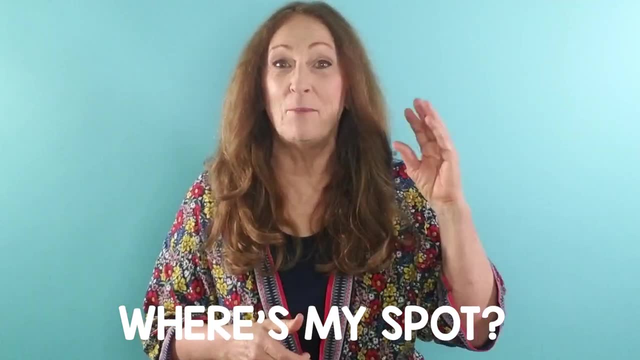 the students have choices of sitting On the first day. I don't care where they sit, I just say come in and I'm singing, come in, come in. you know the ukulele or with the puppet getting them to come into the classroom and just find a spot. 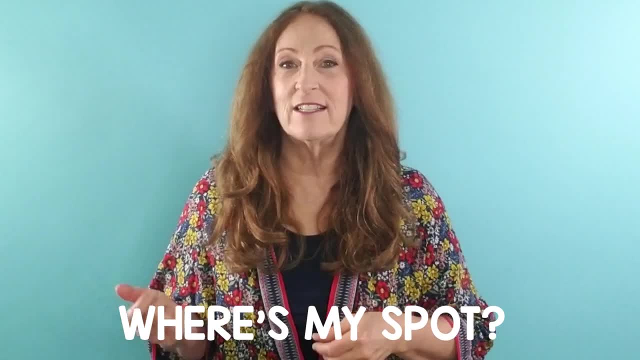 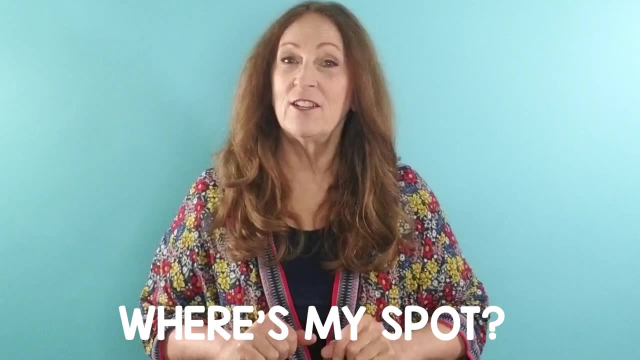 and have them stay standing and sing the song until everybody gets in the room, and then you can teach them to sit down in your choir way, or you can teach them to sit down with the song, and I have a little song for that. it's just super. 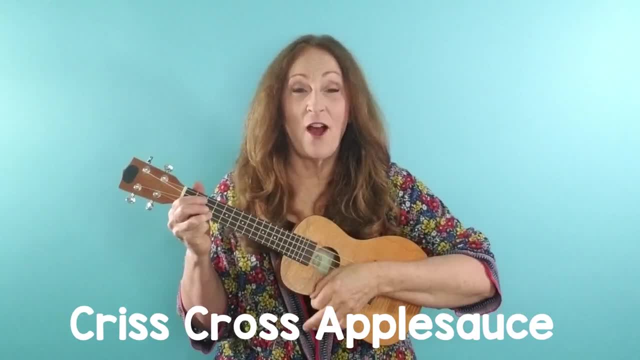 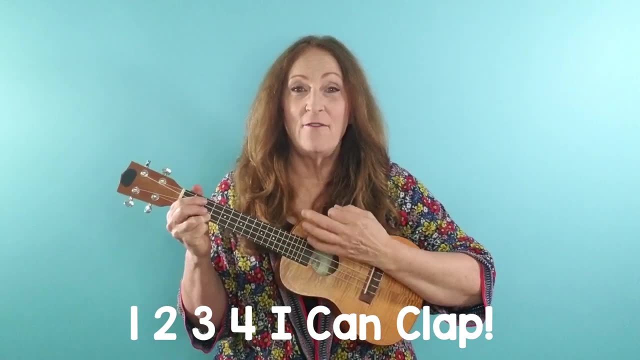 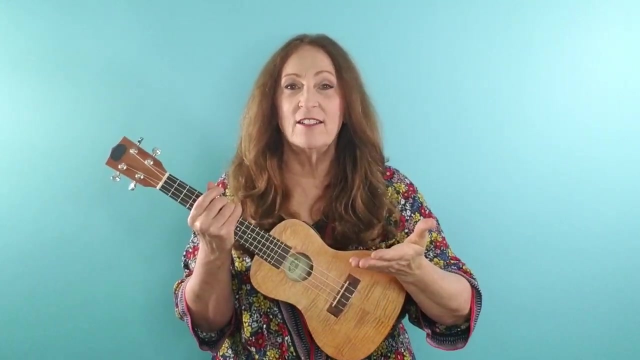 simple. it goes like this: crisscross applesauce hands in your lap, one, two, three, four. I can clap, and I didn't change the chord because I'm just singing the song to them to teach it to them. then I'll put my ukulele away. so 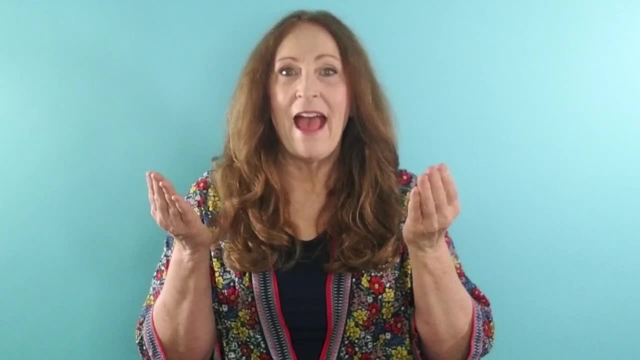 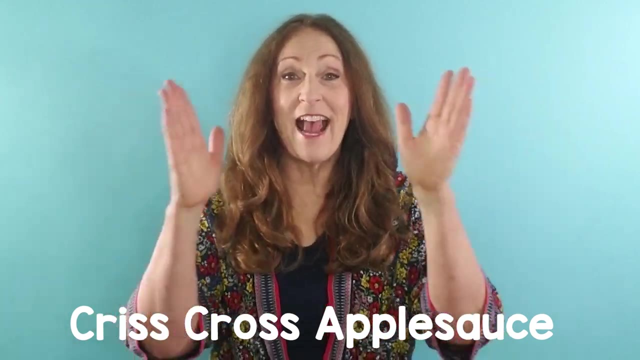 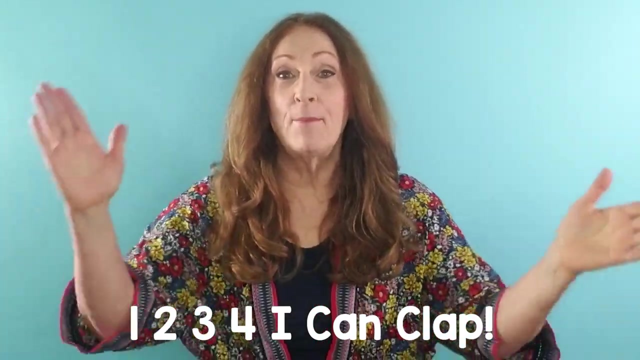 then I teach them how to do the song. and we're standing up and then we're gonna slowly go down. we can be silly: crisscross applesauce hands in my lap. one, two, three, four, I can clap boom, and then we do that a couple times as you're. 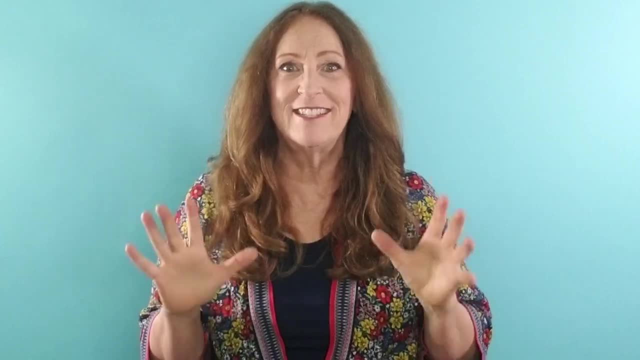 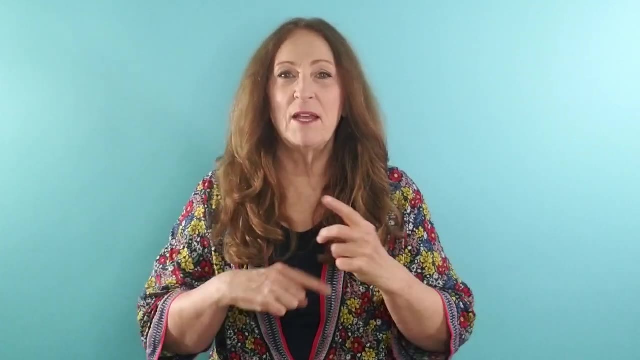 going to try to get everybody to clap boom at the very same time. that's a really fun game. I don't use it all year long because things speed up, but on the first day I'm out of breath and I don't need to move with everyone, so I'm just 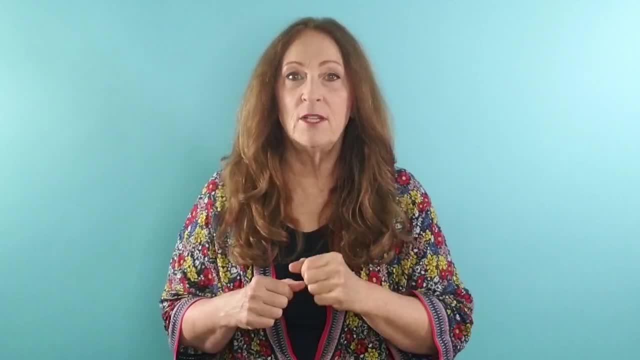 singing the song until they get in, and then I'll get them to do the work. I'm want the kids to watch me. I want them to know that it's important to be quiet when they stand and then when they sit down. it's time to switch our attention. 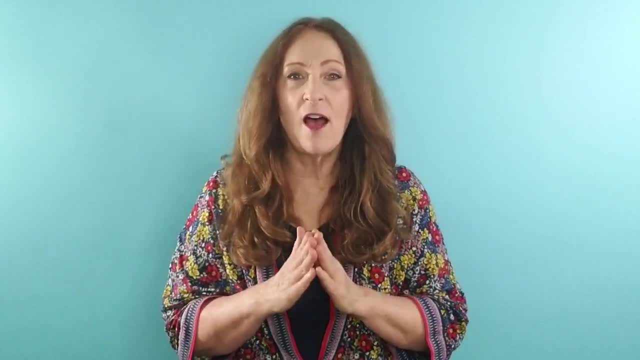 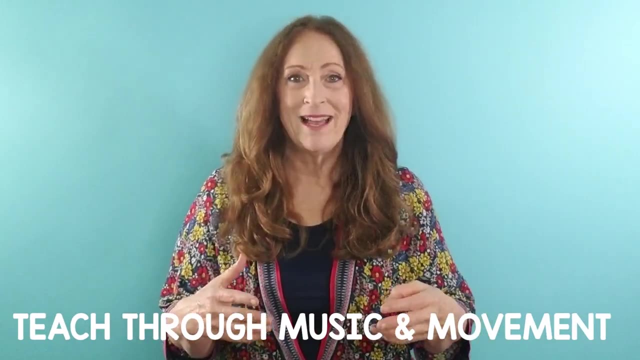 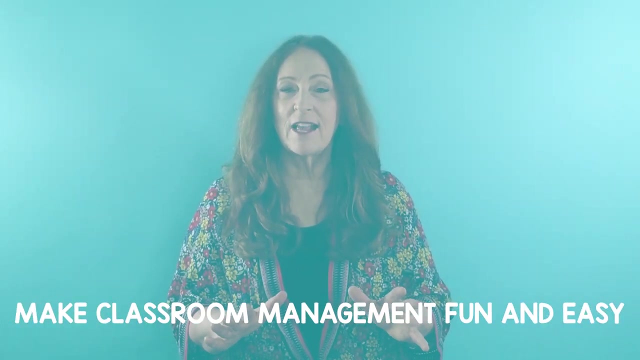 to something different and to pay attention, But I'm not that strict with it all year long. It's just me teaching them these things through movement and through music, to get them to know me and how I want things to go in the music room. It's super important to think of these kinds of things as you teach your. 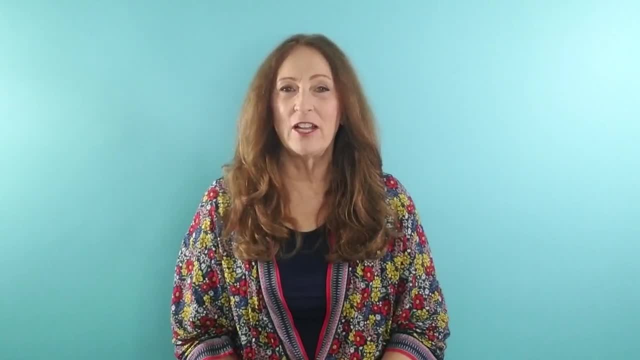 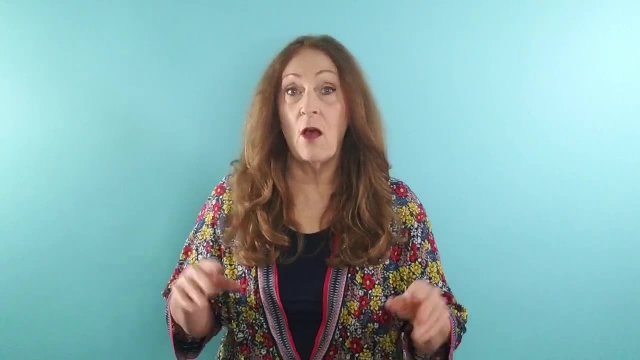 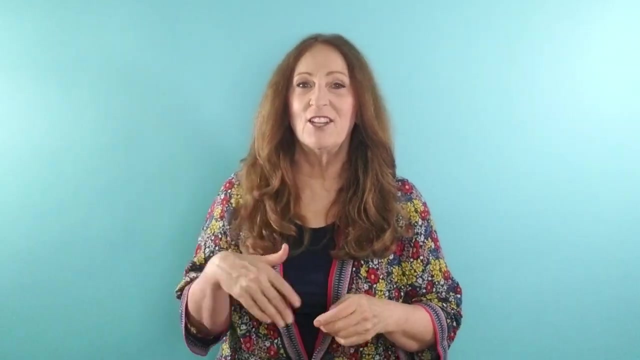 students, because if you begin this in kindergarten, you'll find by the time the kids get to third grade they know, if you just say crisscross applesauce, oh boom, they'll sit down and clap their hands and you can move right on with your story or your presentation or whatever is going on in the classroom. 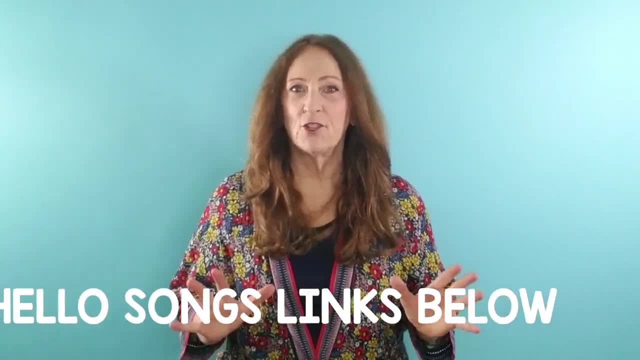 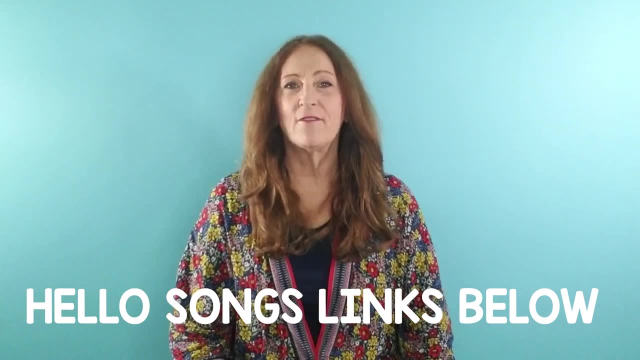 very quickly. If you're looking for some fun hello songs, you can go to the Sing Play Create website or the Teachers Pay Teachers store. I've got the link in the description. I've got some links down below. You'll find some of these really fun hello songs. 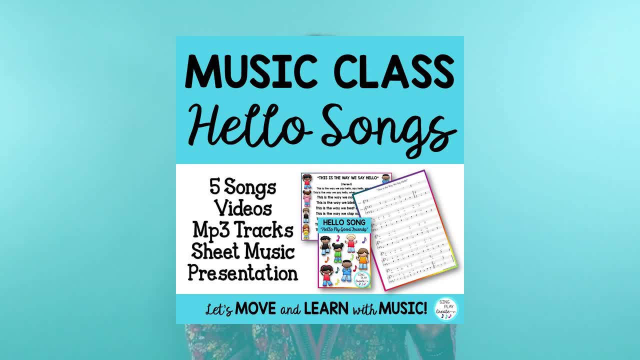 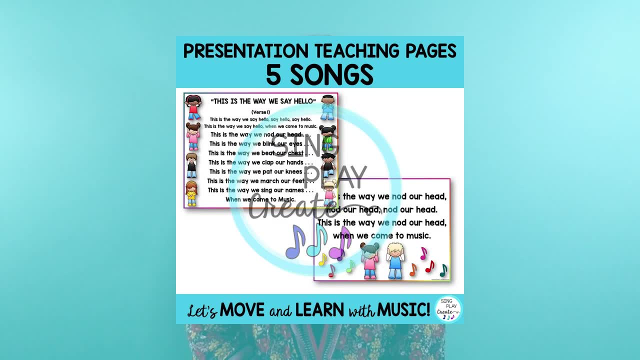 I've got a whole bundle of them because I had a different song for each grade and that way, when they came in, each grade had their own special song that I would sing. I didn't get tired of singing the same song all day, and it was. 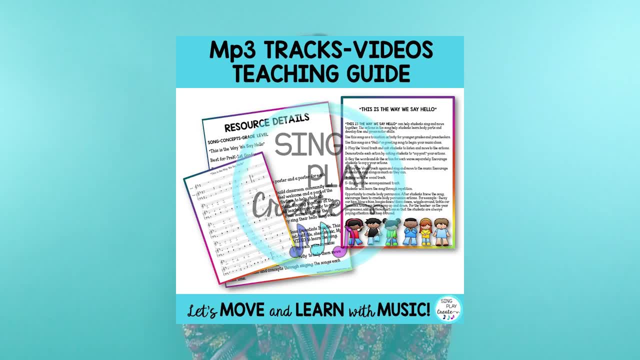 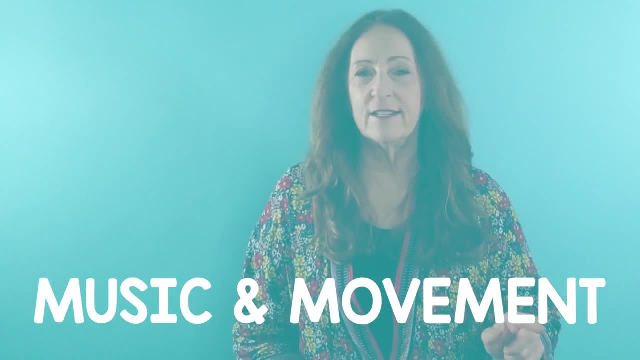 exciting for them to learn a new song. the next year they came back to music, So you can check on those links below After we get done with the hello song. I just want to let you know that I have a free resource that you can use to get into an. 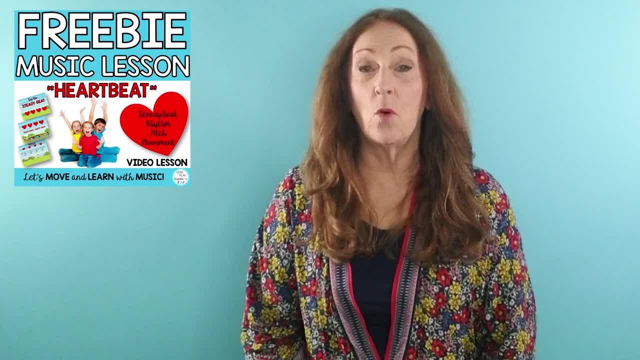 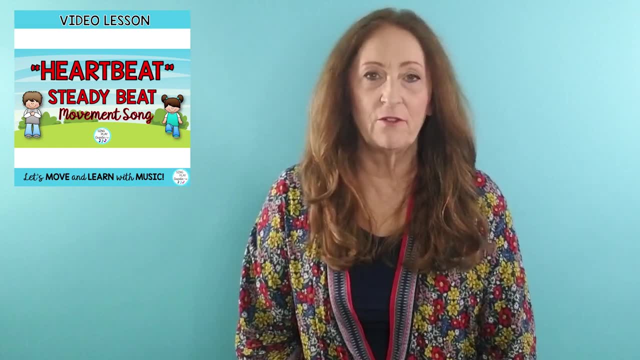 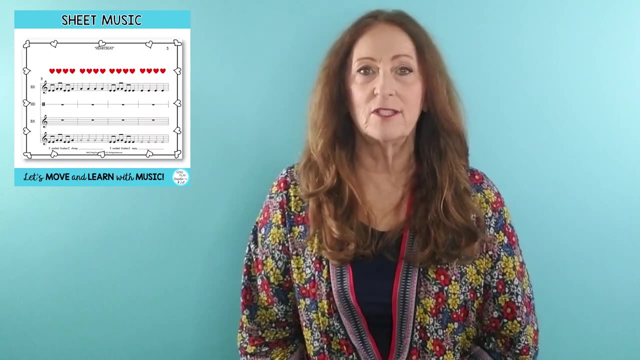 activity. I have them standing up and I do some kind of song movement activity and one that I have. that's a free resource that many people have used. It's got tons of downloads and it's also available in the Sing Play Create free resource library. It's called Heartbeat and it's great for kinder and first. 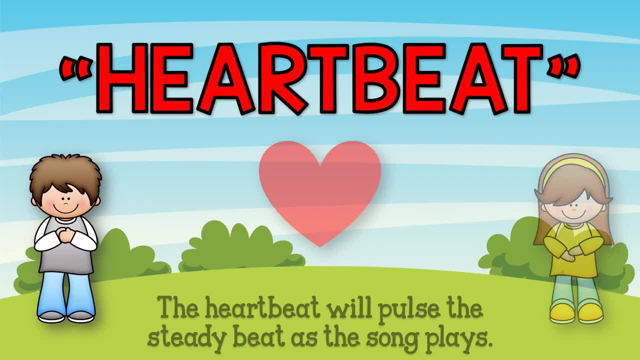 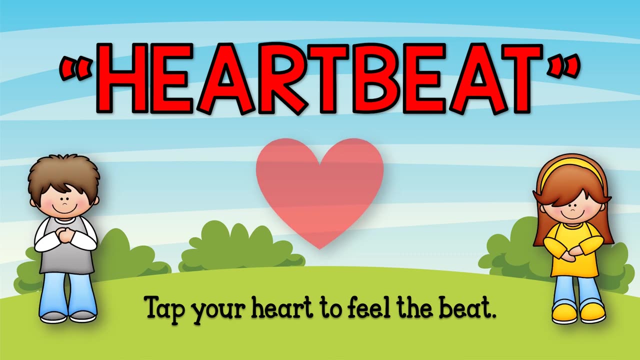 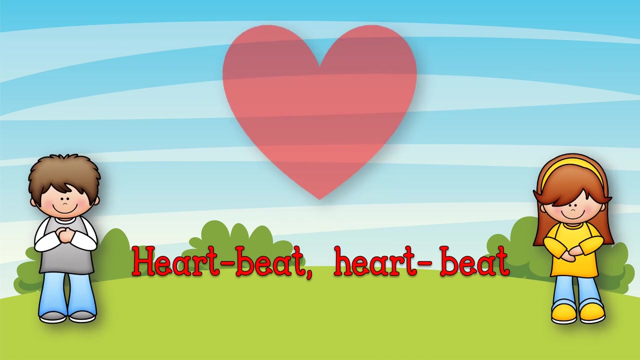 grade, and you can do it with your second graders too. They'll like it. So it goes like this Heartbeat will pulse the steady beat as the song plays. Tap your heart to feel the beat. Heartbeat, heartbeat. I can feel my heartbeat. 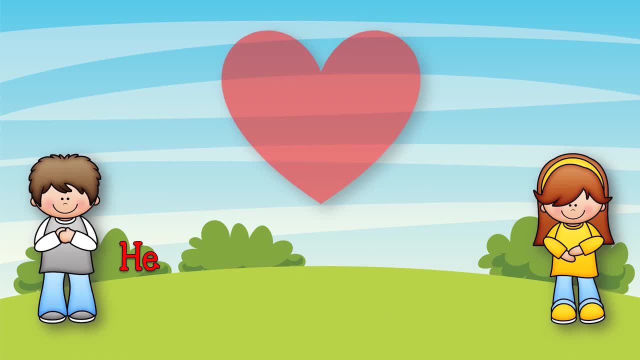 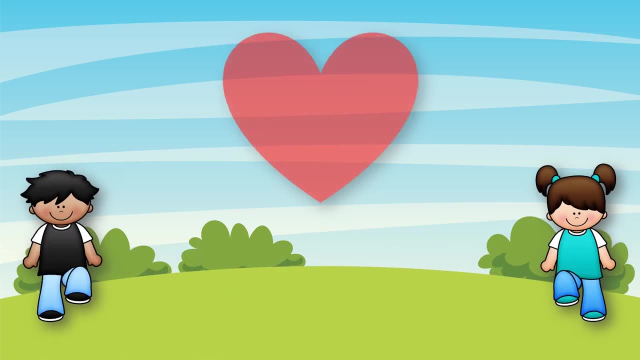 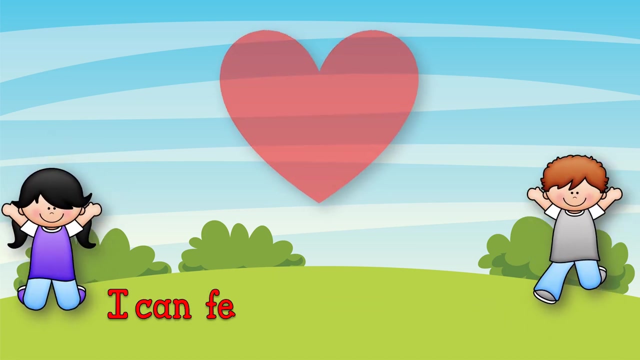 Heartbeat, heartbeat. I can feel my heartbeat, Heartbeat, heartbeat. I can feel my heartbeat, Heartbeat heartbeat. I can feel it when I stomp Heartbeat heartbeat. I can feel it when I snap Heartbeat heartbeat. I can feel it when I jump. 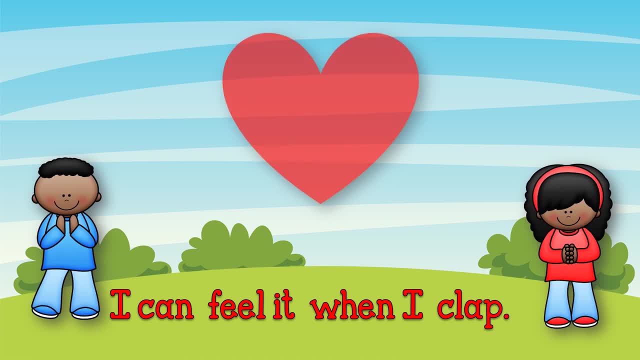 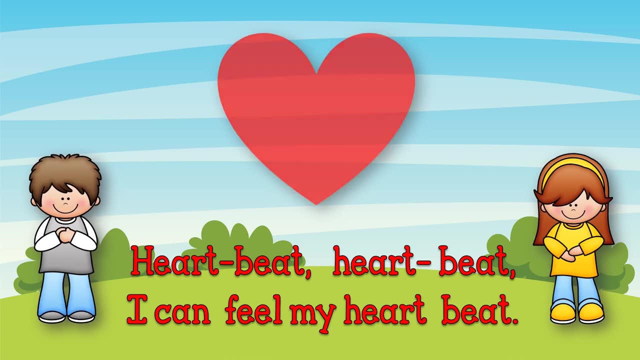 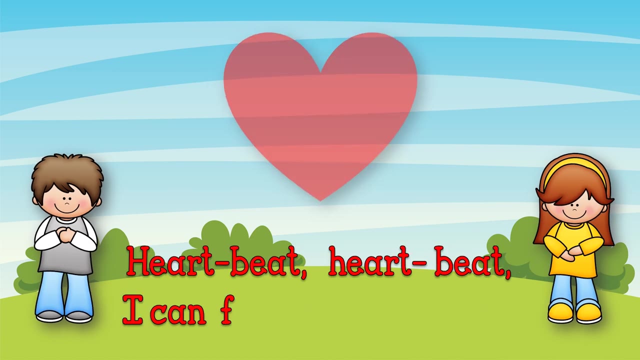 Heartbeat, heartbeat. I can feel it when I clap Heartbeat, heartbeat. I can feel it when I clap Heartbeat, heartbeat. I can feel it when I stomp Heartbeat, heartbeat. I can feel it when I stomp. 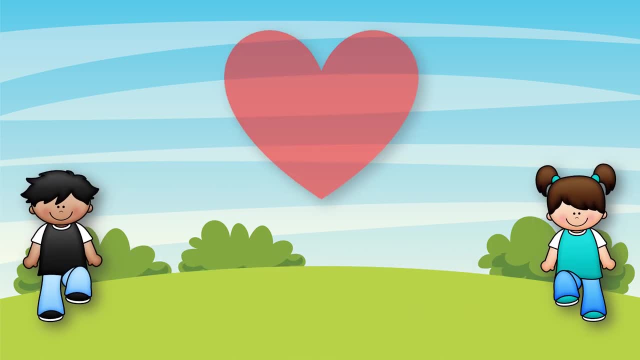 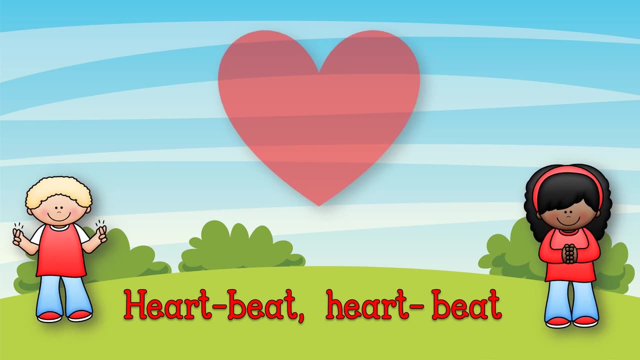 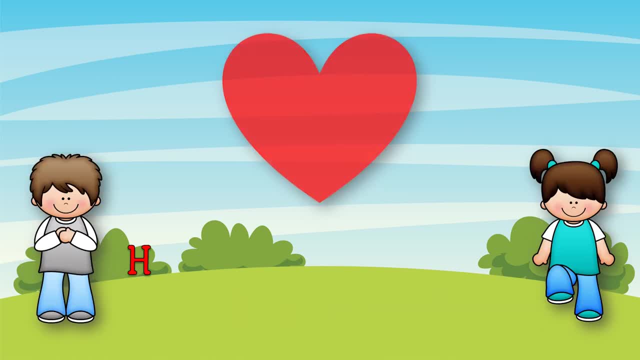 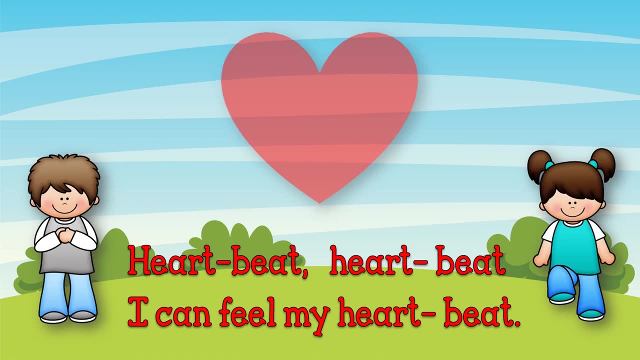 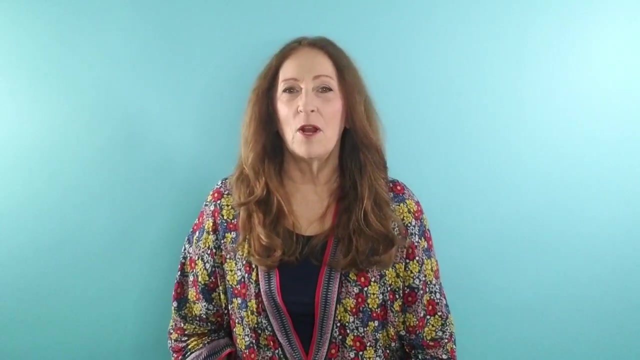 Heartbeat, Heartbeat, Heartbeat, Heartbeat, Heartbeat, heartbeat. I can feel my heartbeat On the first day of class. I'm not gonna really worry about teaching the words. what I'm gonna do is I'm going to just model it. 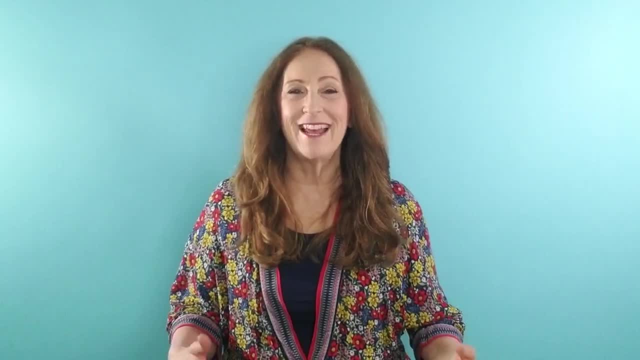 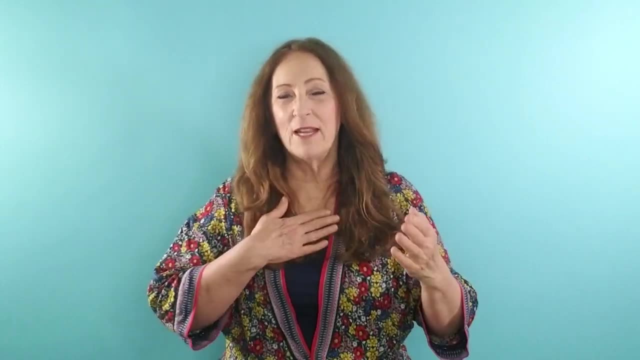 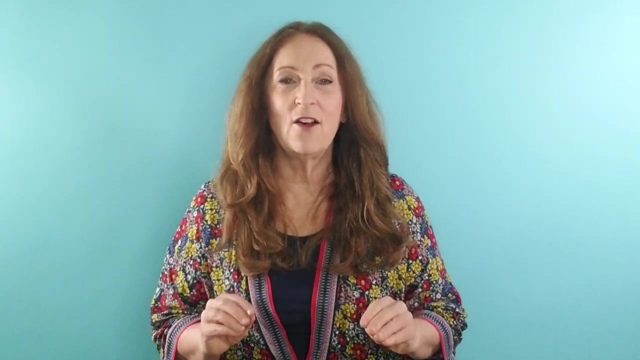 I'm standing in front of the class and I'm modeling it and I'm just smiling and I'm just doing Heartbeat, heartbeat, heart, heartbeat, heartbeat. I can feel my heartbeat and I'm showing the kids how to do the song. it's a very simple song. later I can use that song as a beat and 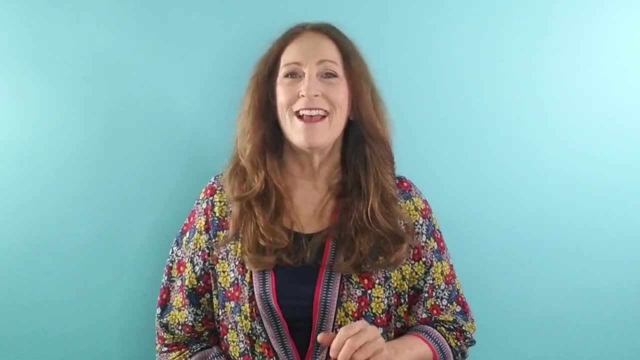 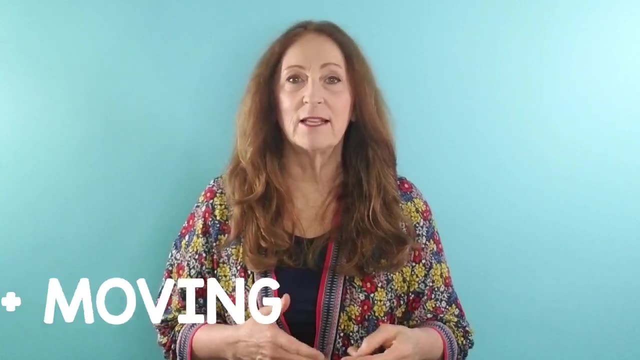 rhythm activity. but for the first day I'm just hoping that this activity is going to make them feel excited about music. it's also going to keep them engaged because I have something on the screen, or at least I'm doing it with the music. they're moving their hands, they're using their eyes, you're using their. 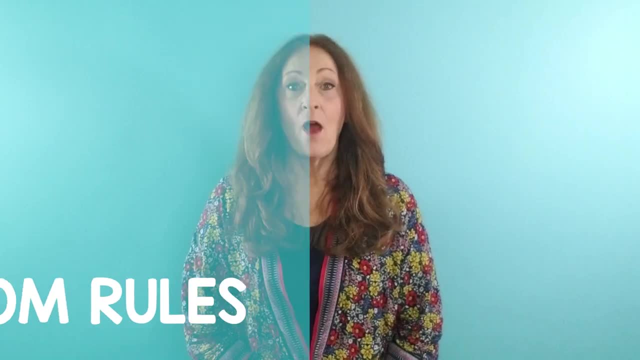 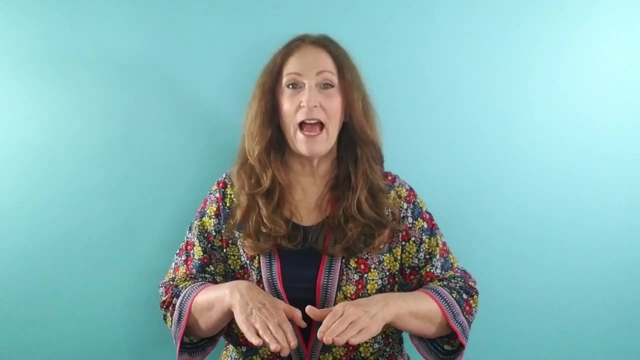 ears and we're making music on the very first day. we say hello and we did a music activity. now it's time, maybe, to sit down, crisscross applesauce hands in my lap and we're going to talk about or listen to or experience some of the 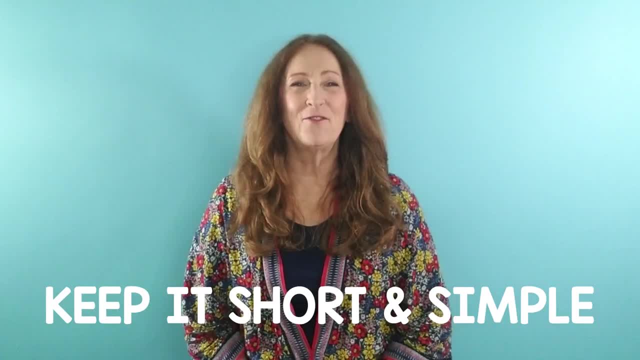 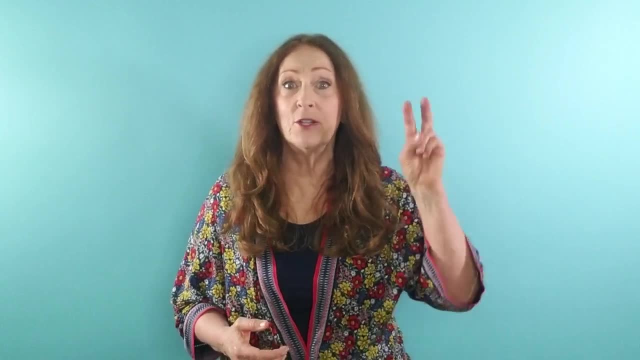 rules and procedures with kindergarten on the first day, I keep it super simple. those poor little guys, their teachers are doing all kinds with them. when I do this, you do this. When I do this, you do this. When I do this back bubble. When I do this, you do this. 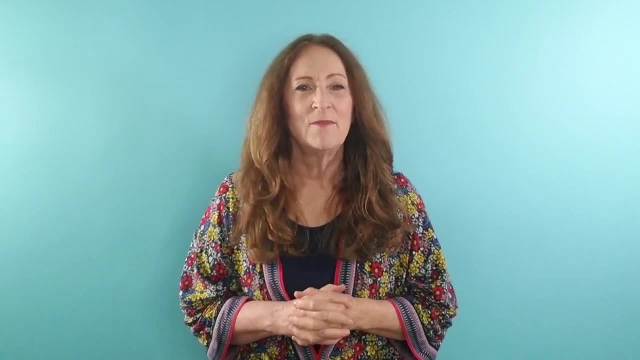 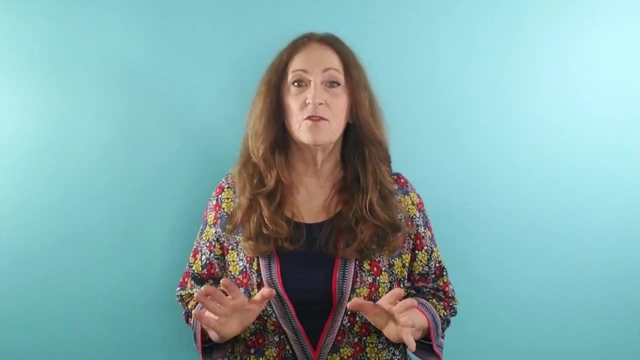 They've got so many things tossed at them on that first day of school that I keep it super simple. So one thing I know that kindergartners always need to work on, and that's following each other in a line. So you can play a little game with them now and you can say: we're going to play, follow. 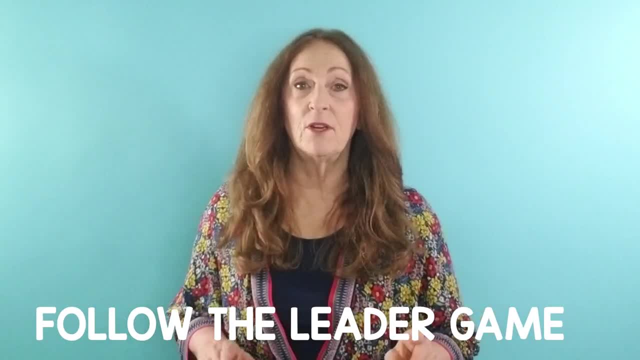 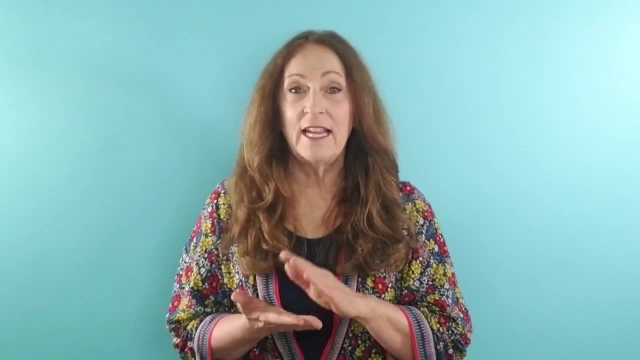 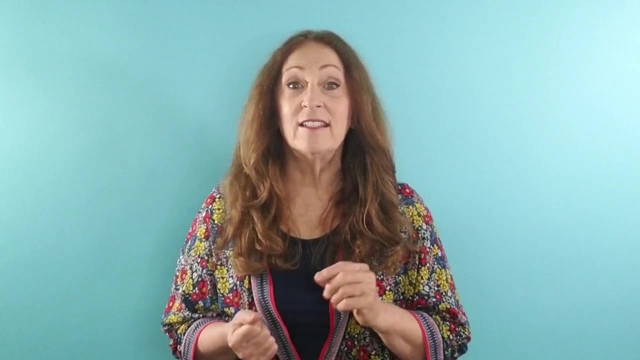 the leader And I have a little song that goes with that. but you can just sing or just play music or use your hand drum and just say: following the leader, leader, leader. we're following the leader in the line, And then I sing that and I'll have them follow me. 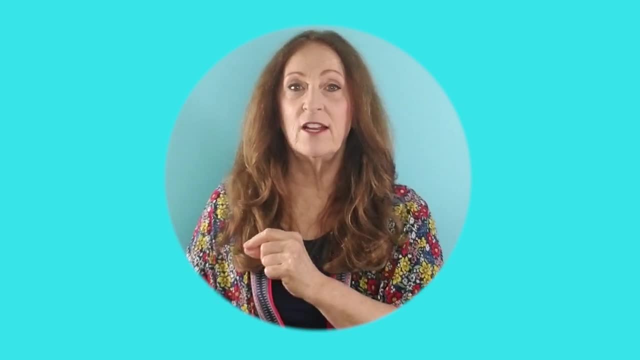 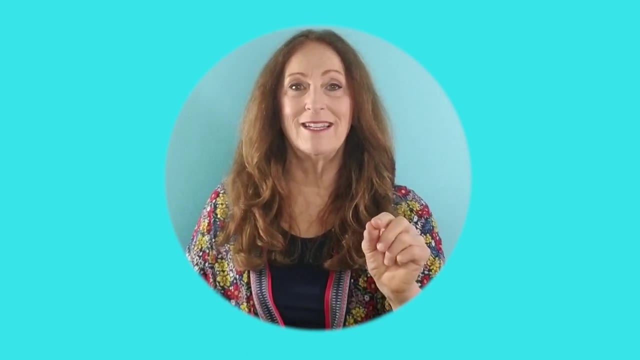 And I just walk in the circle. I don't try and do anything crazy on the first day, And this is when I teach my students where we're lining up, because what I did is I had the circle start where the door was and then they walked around. 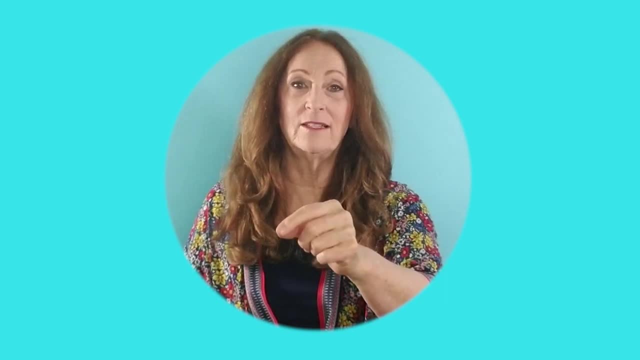 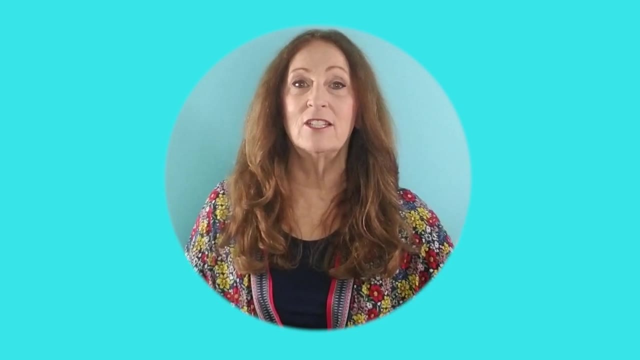 Okay, Okay. And then, of course, the circle ended where the door was and they would stop. there had a special dot for them to stop And then they would stop in line and then their teacher would come and pick them up And it was just easy for me to make the line as part of the circle. 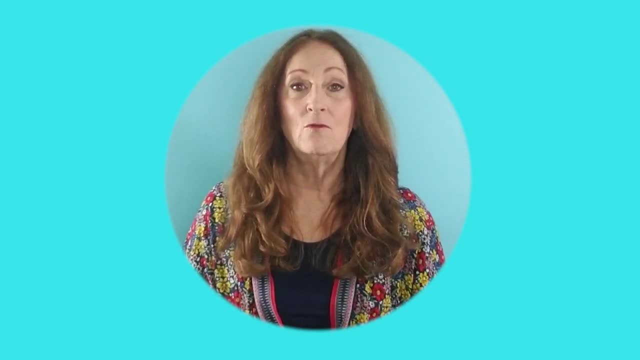 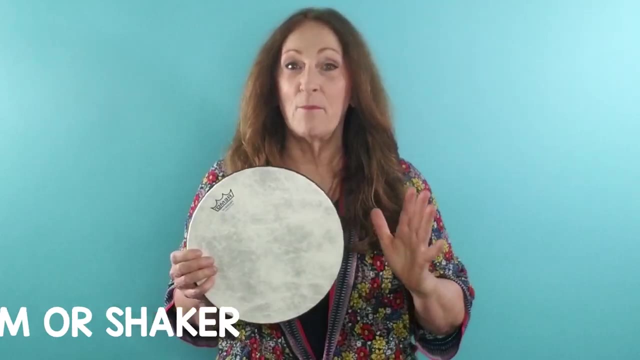 That way they didn't have to have a different place to line up or running here, running there. It was just part of our circle. But we always walked around the circle and we practiced that. There's a couple of fun ways that you can play this game. 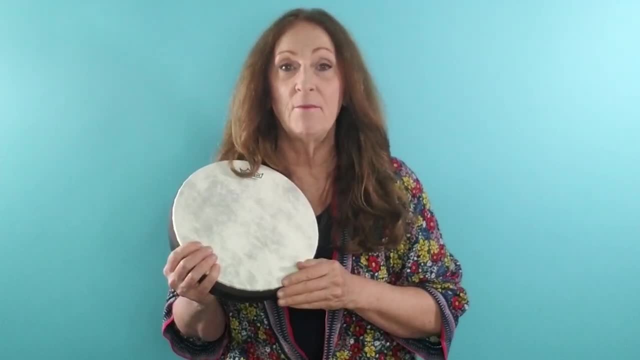 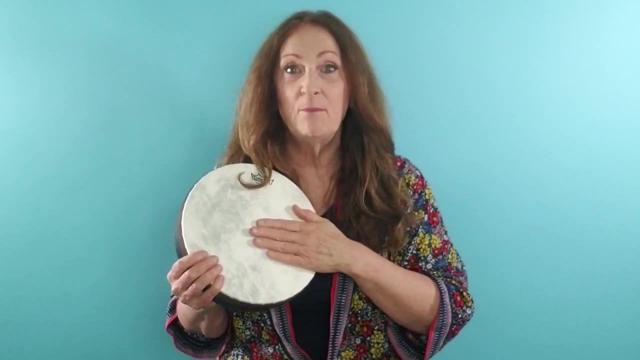 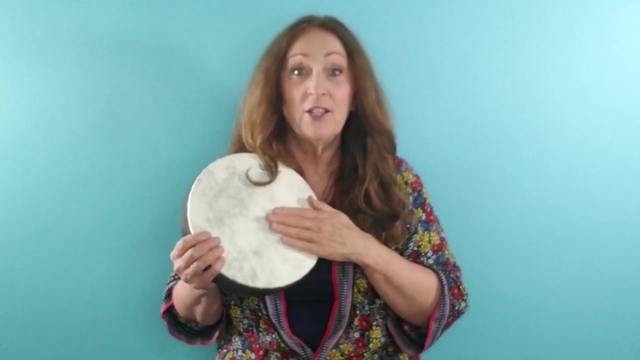 You can follow you and you can play the drum and you can change the tempo Following the leader leader And make big steps. you know following the leader, Then you can speed it up. leader leader following the leader in the. 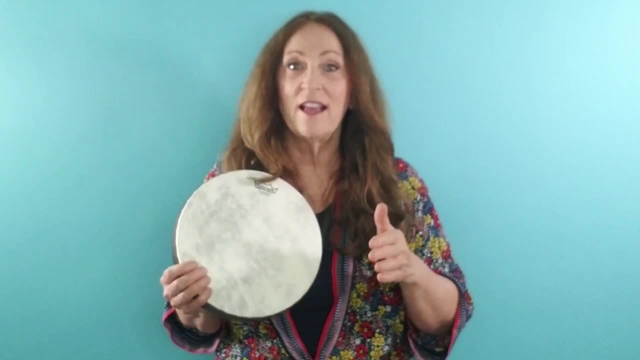 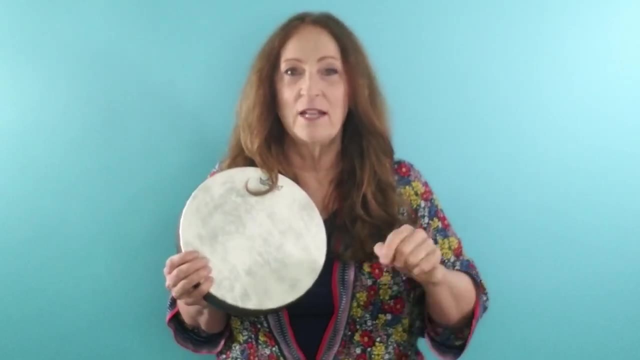 See if they can stop Line So you can switch that up. but depending on your grade, K-2 is going to get it and they can have a little more fun. You might be able to wiggle around a little bit and switch directions and go back and 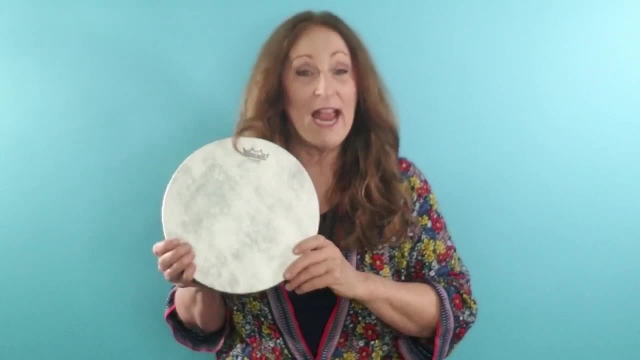 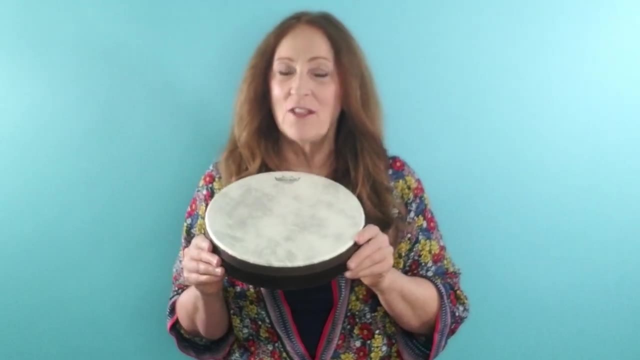 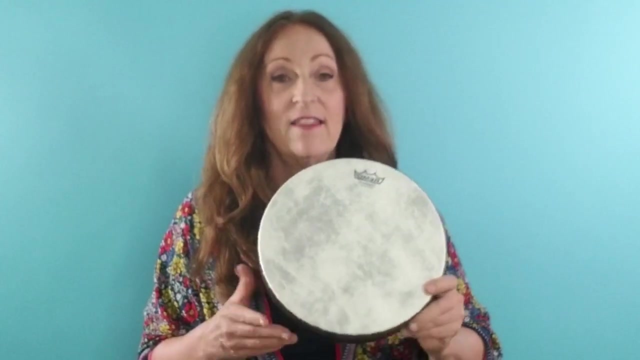 then have just the kinders, just stay in the circle. But a hand drum playing along with you or a shaker or something, will really help the game move along and it makes it fun for the kids. And then you can say: and later you're going to get to play a hand drum, just like this. 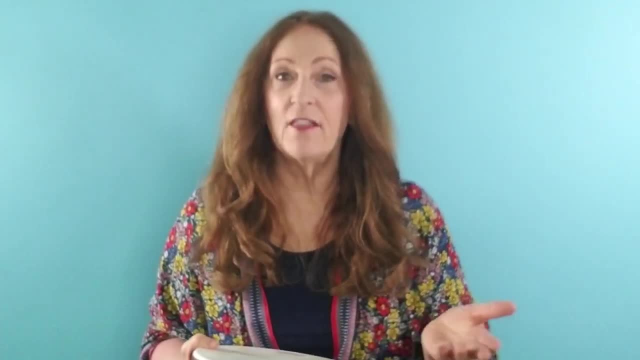 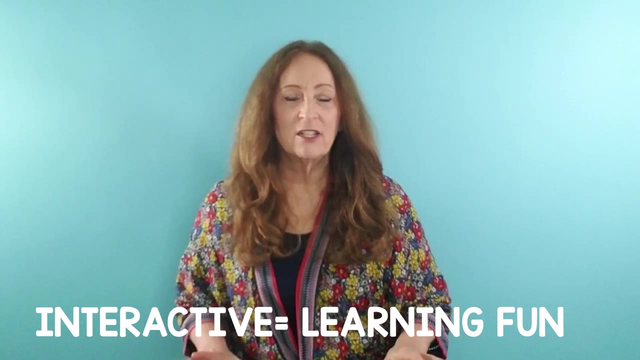 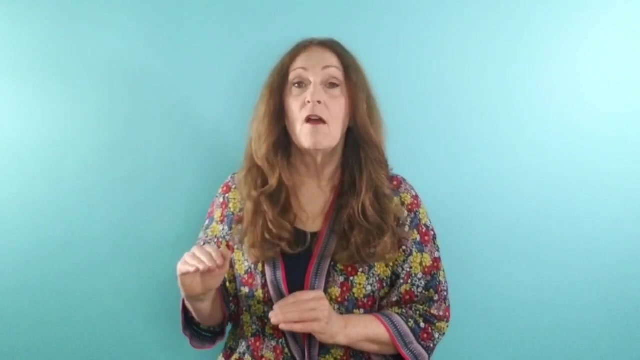 And then that's a really great way to just share another thing that's going to happen in the music room on the very first day. I really like to use movement or actions or something interactive to teach the rules, And so I do have a PowerPoint and I will go through the rules for sure on that very first. 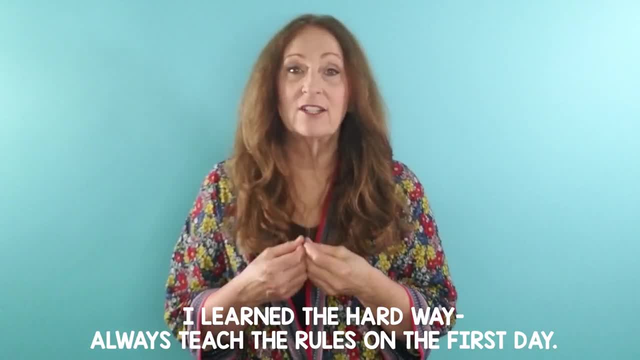 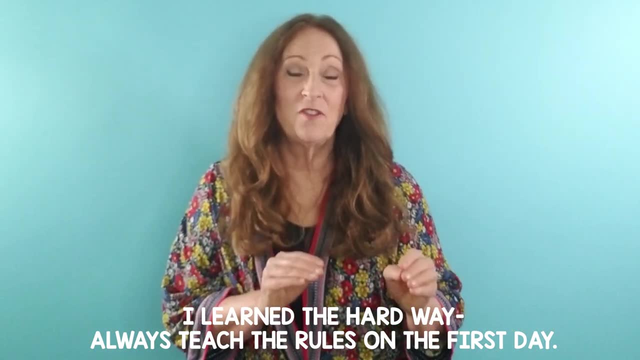 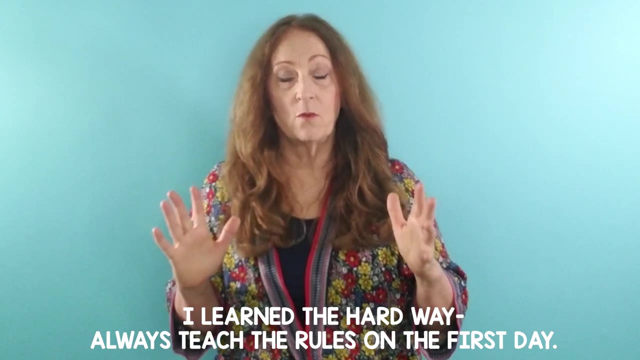 day. Sometimes I have done this. I actually have not done it or I've skipped over it or just kind of. you know, I did some of those procedure things but I didn't really go through the rules of the room Because I was thinking, oh, the kids are so overwhelmed. 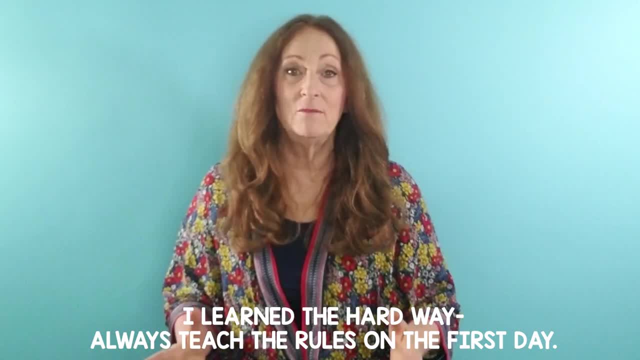 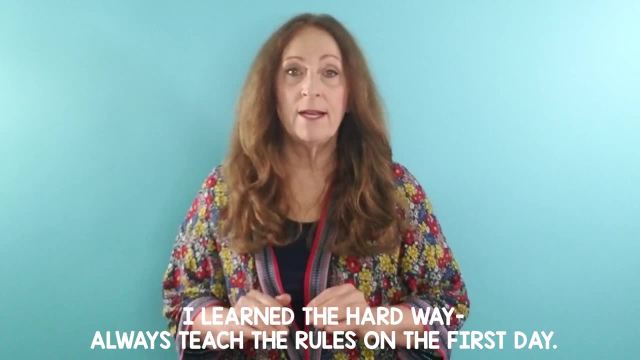 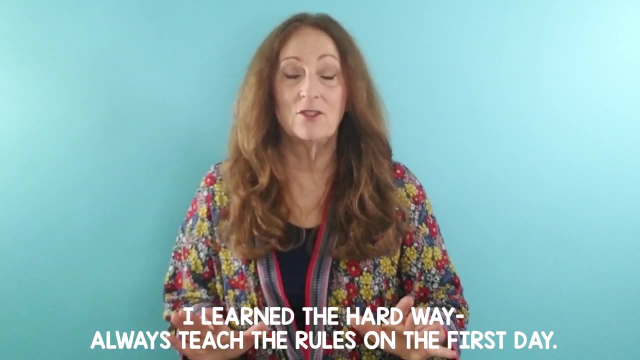 There's so much to do and I just want them to have fun in music. It's a hard lesson to learn, but I did learn that it is really important to take my time. you know, pay attention to the flow of the students, if they're like, if it's right after. 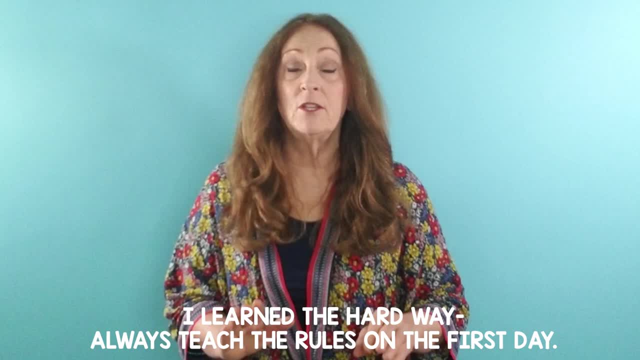 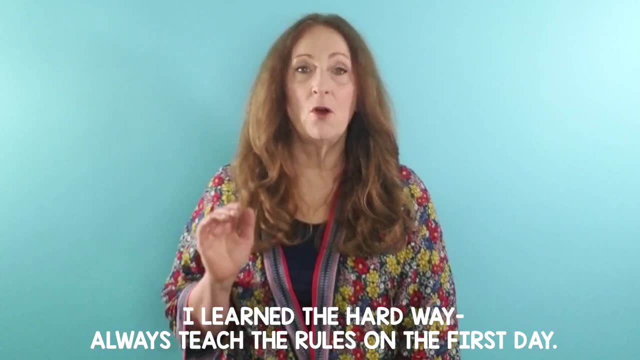 lunch and they're really tired, then you know, maybe you'd shorten it a bit, but you'd want to go through your rules on the very first day, whatever they are. I always had mine posted, So I just read them right from the bulletin board. 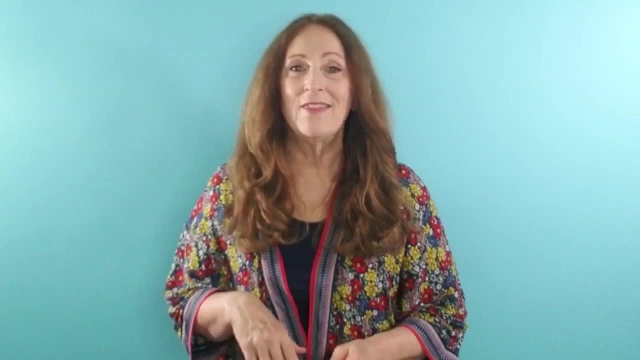 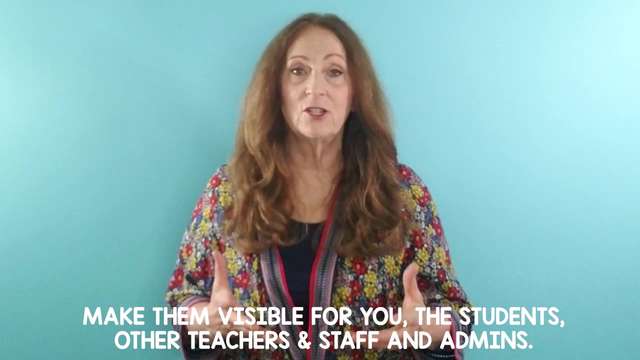 That way, all the teachers could also see my rules, And that's a really important thing, because you want them to back you up on your rules and you want them- all the other teachers that come to get their kids- you want them to know that you do have rules in your classroom. 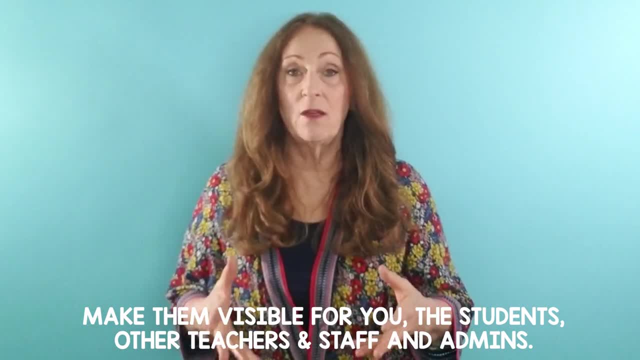 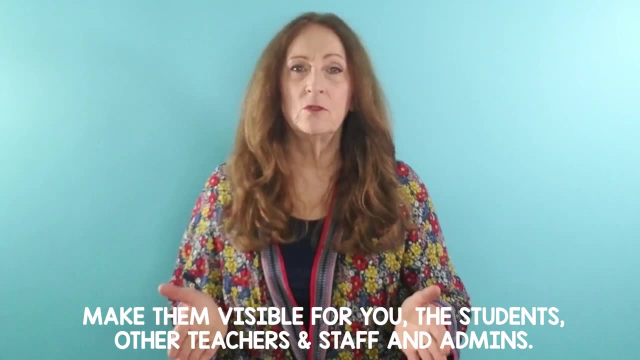 That, no, they just can't come to music and run around and do whatever they want to That. we're here to learn too, And so we have rules that help us learn. So, whatever your rules are, That's what we're here to learn. 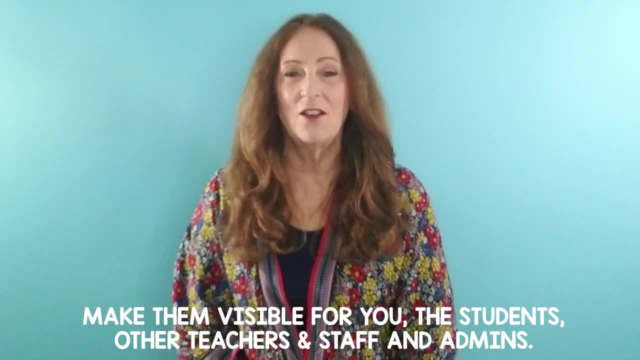 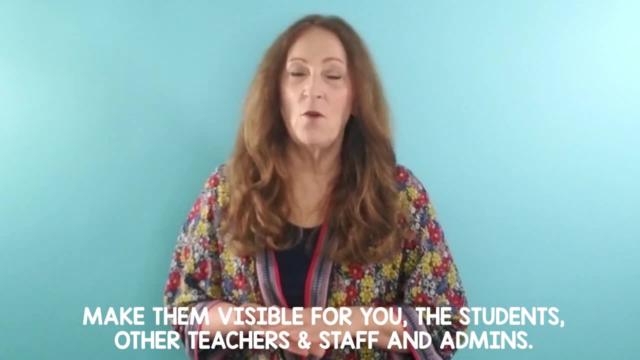 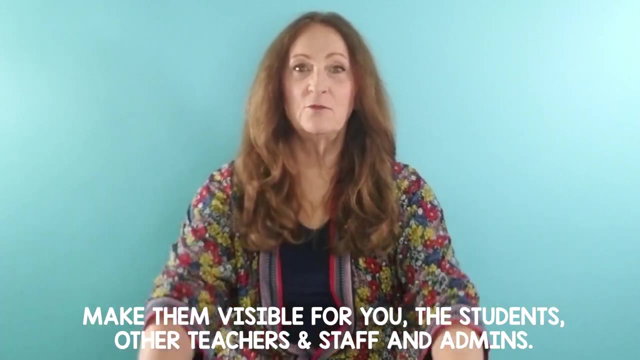 That's kind of up to you, but I do feel it's important to communicate those the very first day of class. and if you can do it in a fun way, use the puppet, do it in a chanting voice, do it. rule one. rule two. rule three: knees. rule four: 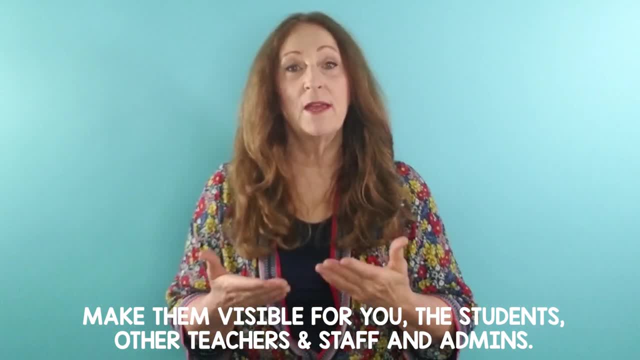 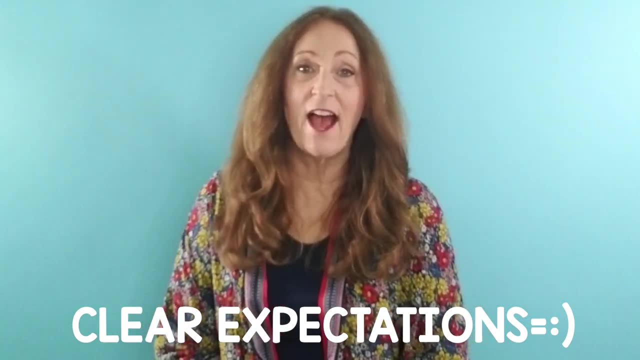 You can do something like that where you can use the body to help them learn the rules. Keep it simple, but be clear and set those expectations on the very first day. I have found that difficult. I have found that to be super successful in classroom management. 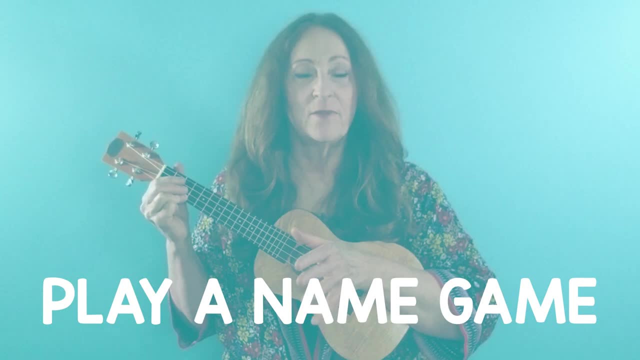 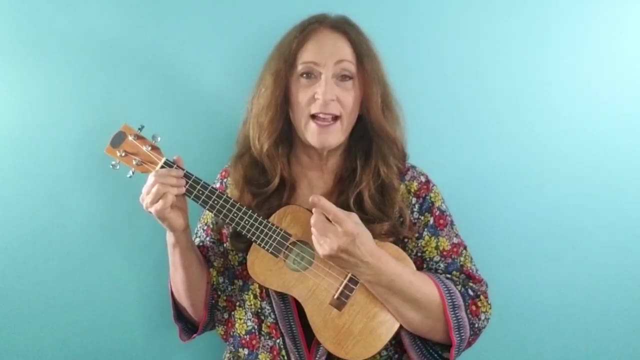 It's the very first day of school, or the very first day of music class, and to me now we're getting to actually the most important thing. We've sang a hello song to welcome our students in. We're smiling, We've greeted them, 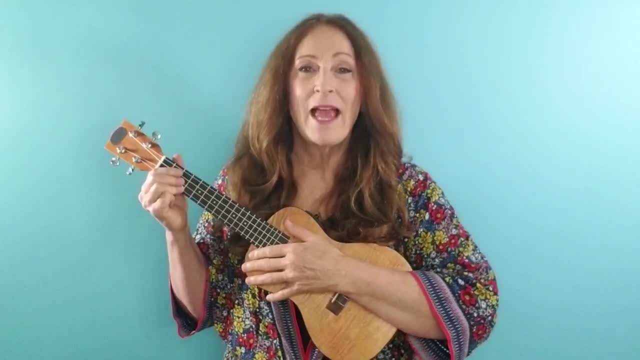 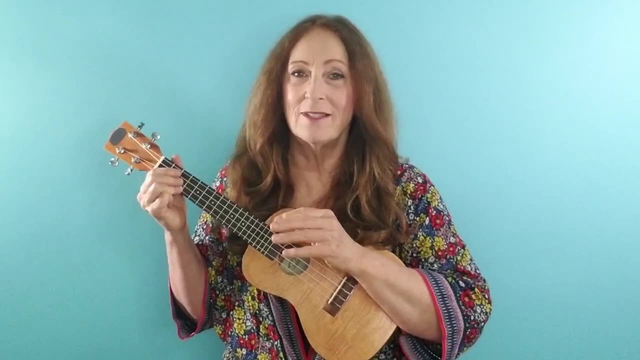 We have done some procedures and rules activities, and now it's time to play a game. I like to make sure I get in some of those procedures and the rules, And then I might just have maybe 10 minutes left of class, or I might have 15.. 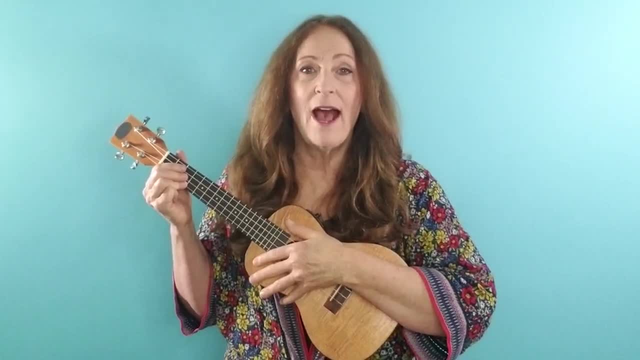 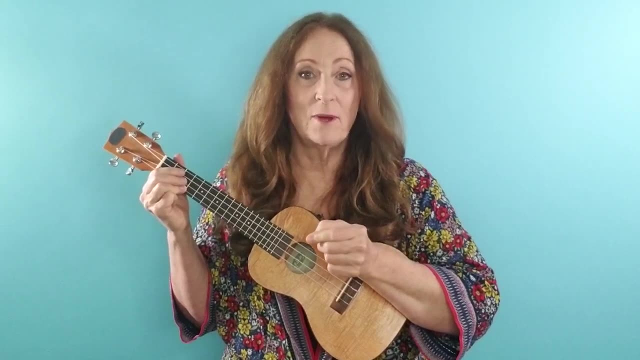 It just depends on how those other things have gone. So I have a game and I'll tell them. you know, we're going to play a little game and I keep it really short so I can get through everybody's name And you can do it in less than 10 minutes. 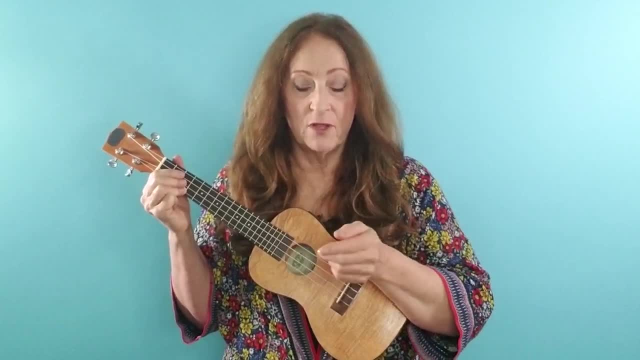 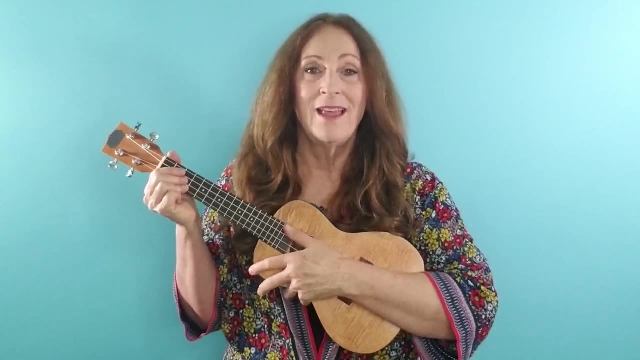 So I have a class list and I'm just going to put the class list in front of me because I haven't worried about where everyone is sitting on the very first day, especially with kindergarten. And I don't know about you, but at my school usually we didn't have all the correct lists. the very first day. So instead of getting all upset about it or, like you know, anxious about it, like what is what I would do? then I realized, you know, just use what I have, And if there's five kids that are on the list, then I can work that out during the game. 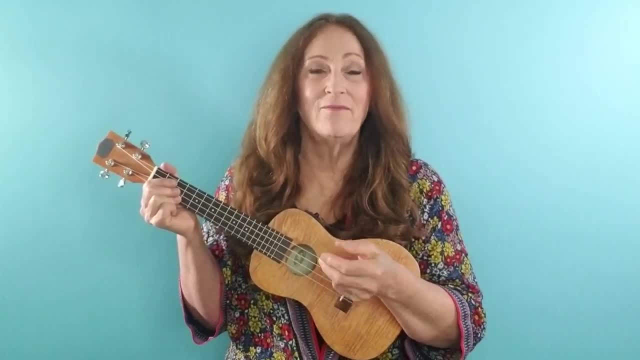 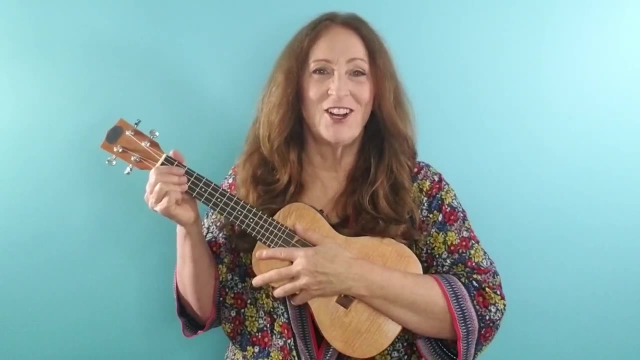 And I don't have to put them in a spot the first day. I can do that even on the third class time. I can wait till we get everything set And then I can make my seat charts. So now we're getting to the meat of the music class. 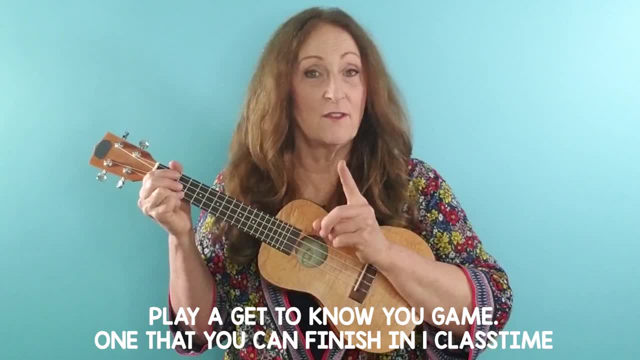 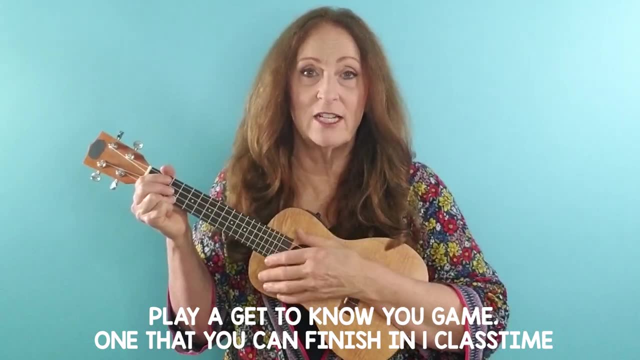 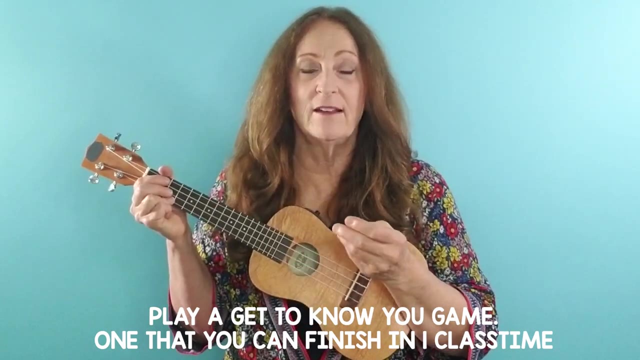 And that is an opportunity to get to know the students on the first day and make them feel included, Also to try and make a connection with them, a very personal connection, And one way to do that is to use their names. So I really, really support and urge you to use some kind of name game. 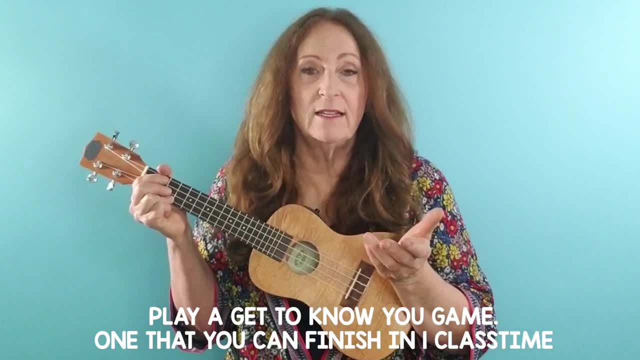 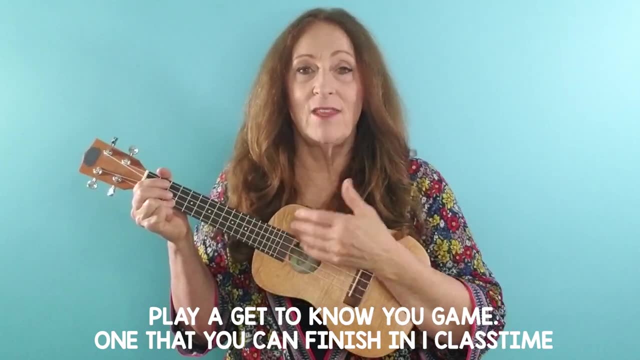 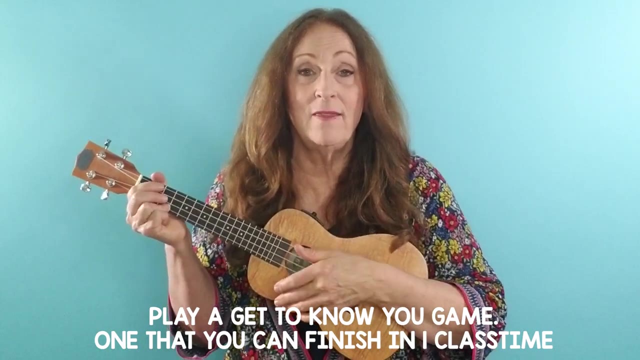 And I think what happens is like what happened to me is when you're first new, it's so overwhelming. But all I did was use the class list. I didn't put everybody in a seat chart. I decided that it was more important to just say their name and they can wave to me or 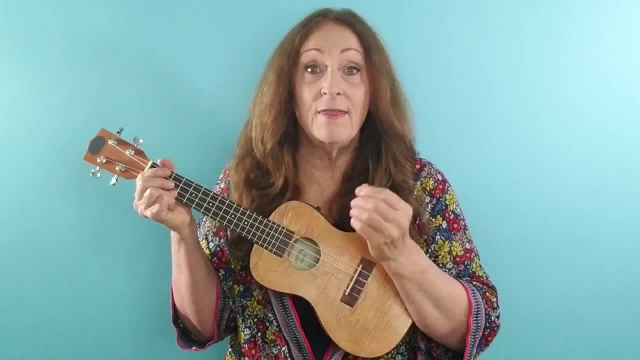 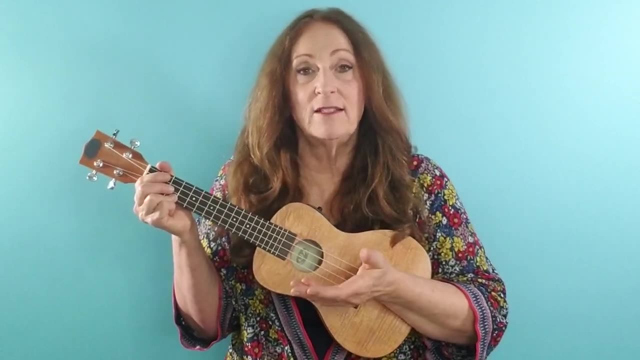 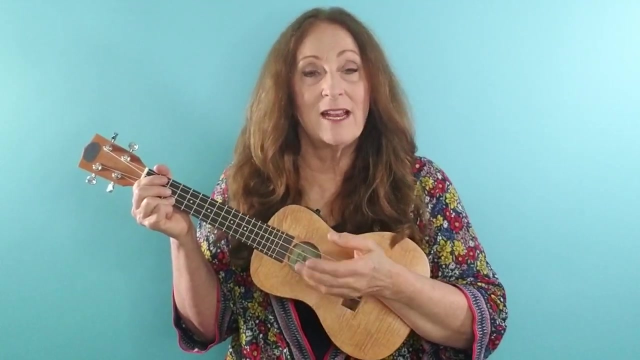 the other kids will point to that kid if they're really shy, And then I could make some eye contact with them and verbally saying their name on that first day And I found that to be super effective. They would know who I was, They respected me because I knew their name and had taken the time to learn it. 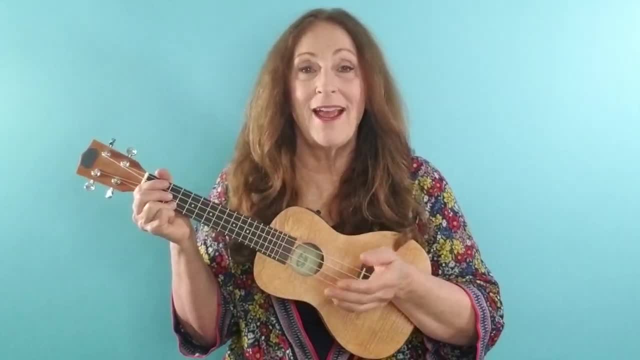 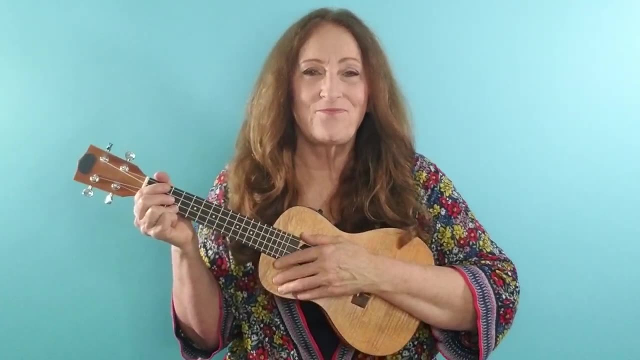 So it's just something I feel has been really important And I also feel like it was super successful as far as classroom management goes, to learn all those kids' names. So you can do it a lot of different ways. Here's just one idea. 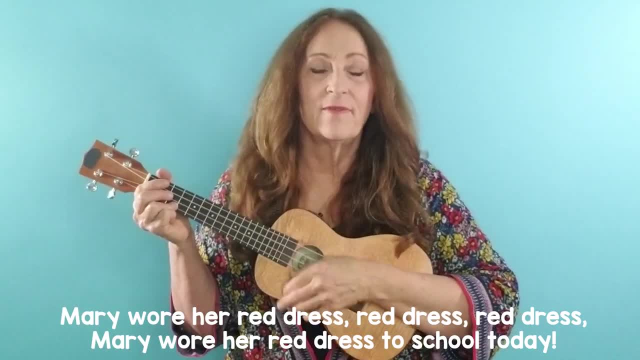 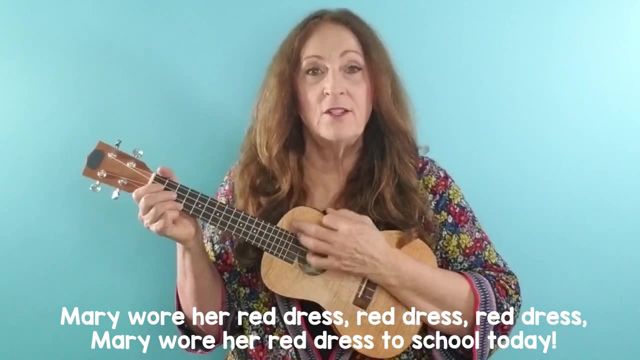 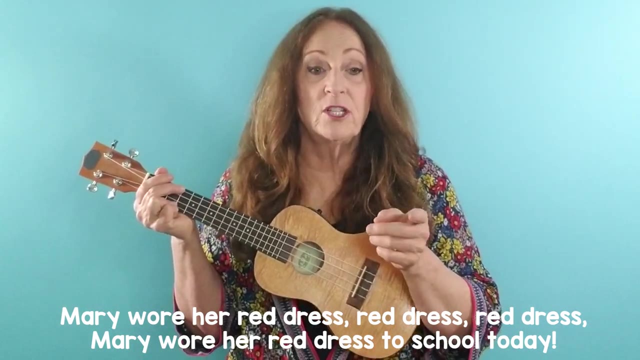 I just took the song: Mary wore her red dress, Red dress, red dress. Mary wore her red dress to school today. So I just took that and I would just change the kid's name And I would just look at what they're wearing and say green shoes, green shoes, 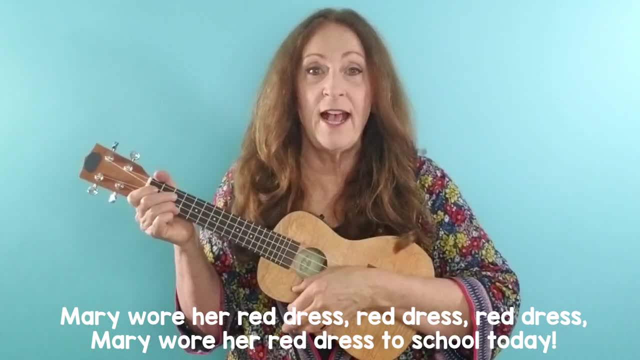 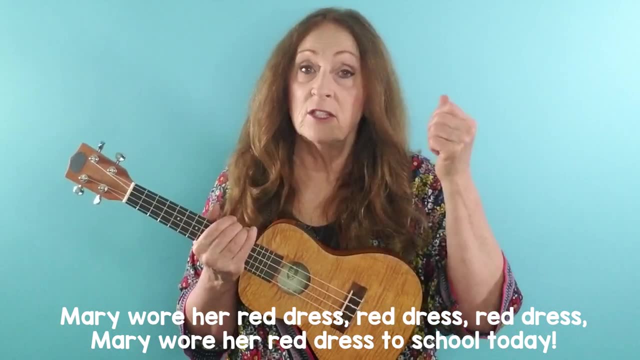 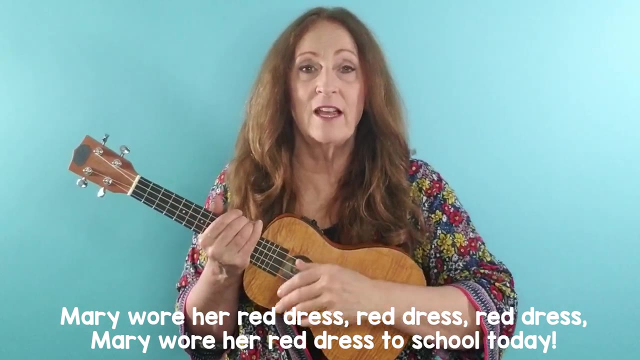 Johnny wore his green shoes to school today. Inevitably on the first day I might not say their name right, or maybe they go by their middle name. So I had a pencil handy, I had the list on a clipboard And I just took the time right then to fix it and then I would sing it correctly to them. 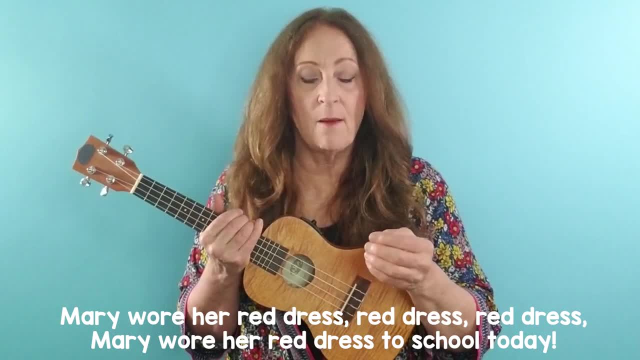 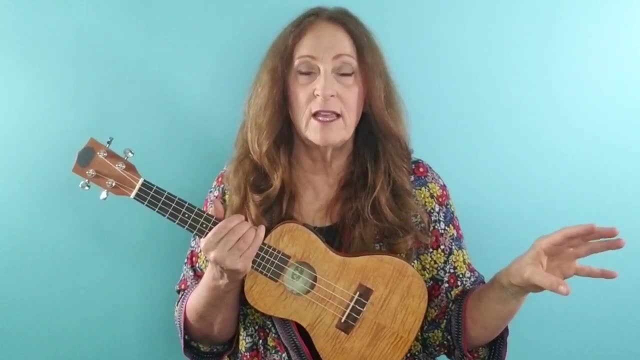 And they just thought that was really special, that I would stop write their name down, pay attention to them. I wasn't in a hurry to go on to something else that I just think we really had to do. that day. My most important thing was to sing their names. 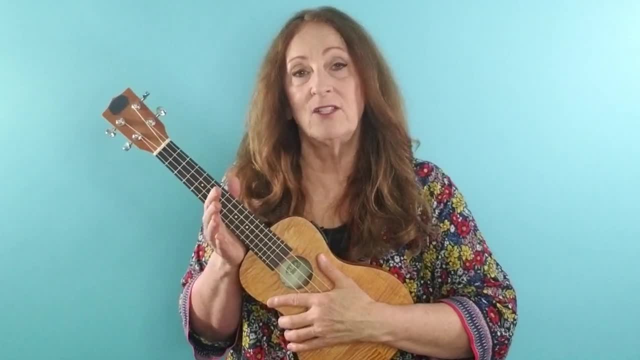 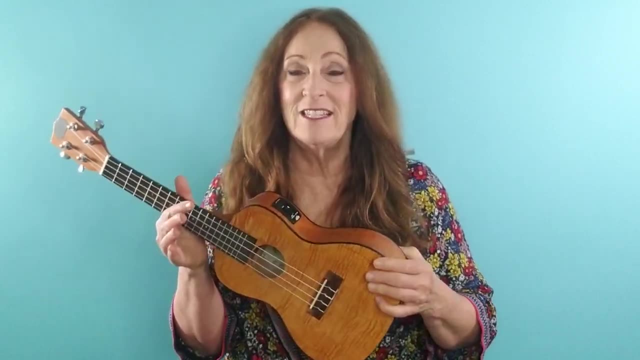 I've done it with a hand drum. I just like the ukulele too. I used to use the guitar. The guitar is bigger, It's a little hard to maneuver, It's easier with the kids, So this is just easy to grab and I would use the ukulele to sing the song. 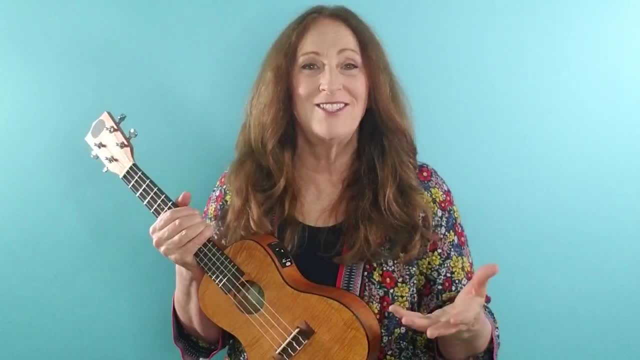 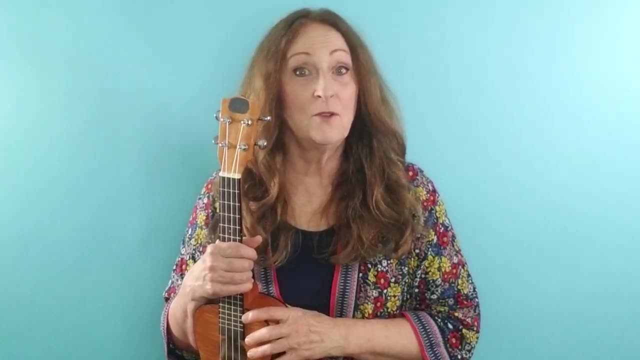 Also, if I need to, I can move around easier with it if I need to. So I hope that you will find a name game or a name song that works for you so you can get to know your students on the very first day and make those important relationship. 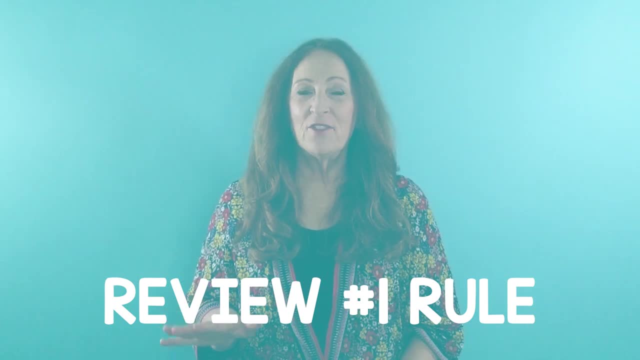 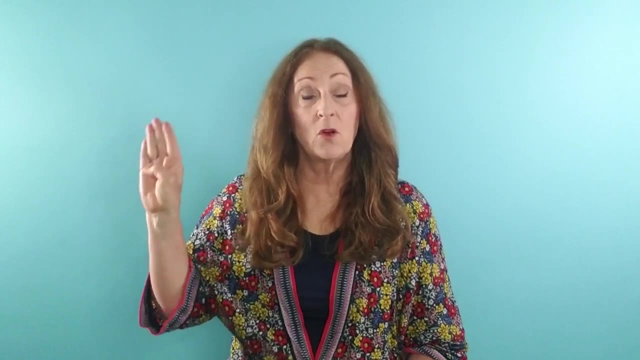 connections. So if we've gotten through the name game, it's always a good idea To make sure you've taught all those rules, but if you went quickly through them and there's one that you think you really want to focus on now, now's the time where you can bring. 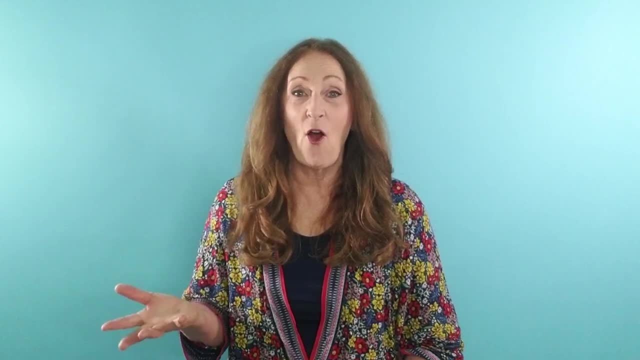 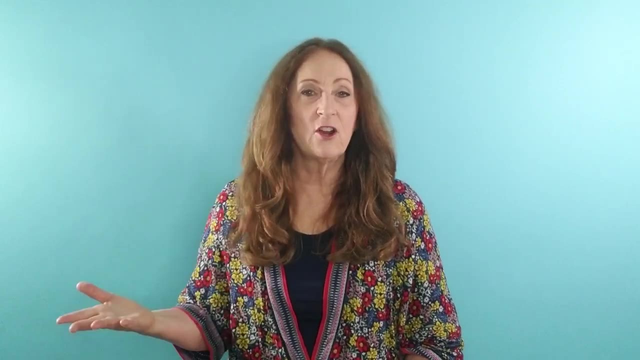 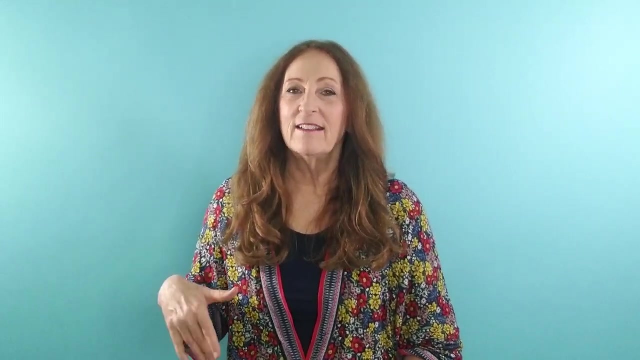 it in, And one of the rules- I think that is the hardest to teach- is keeping our hands, feet and words to ourselves, And you can teach it all year long and you may never be successful at it happening, but, like I said, I think it's important to share. 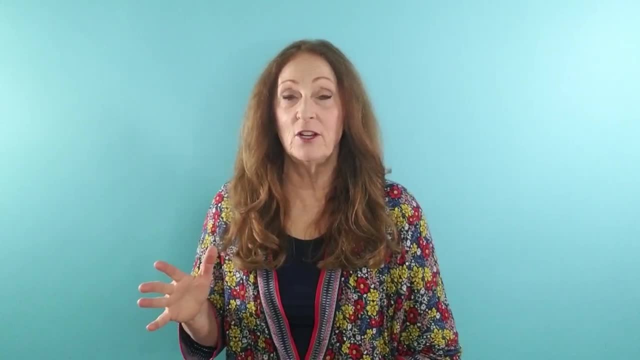 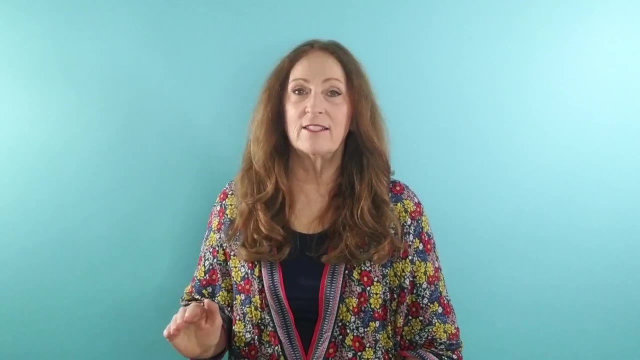 It's important to share these expectations at the beginning of the year because, even if you get 60% of the students who will follow it, that's going to help you keep the class going. So you can do a fun thing like you can have the puppet come back out and say: hello, boys. 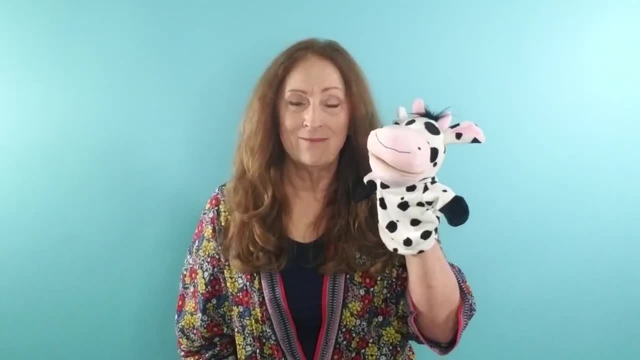 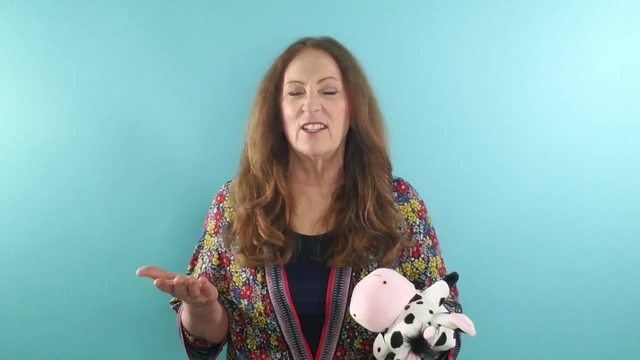 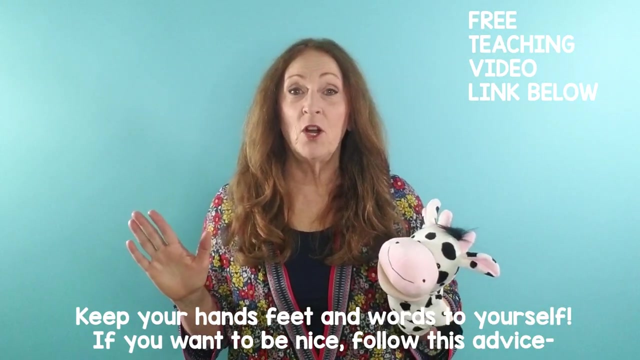 and girls, I want to talk to you about something really important. You could do a little puppet thing. You might have a special song. I have a song. It's easy to learn If you're happy and you know it. Keep your hands, feet and words to yourself. 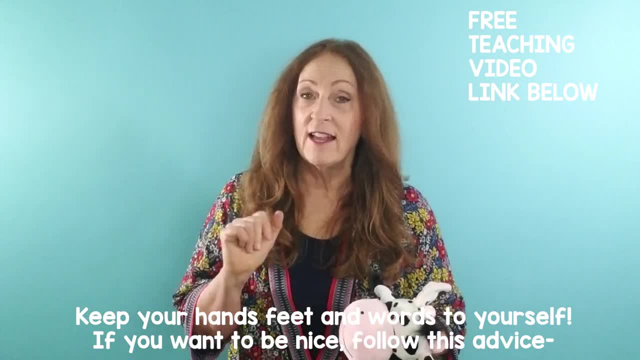 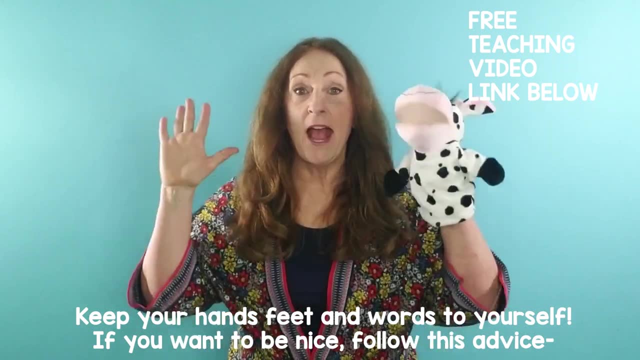 If you want to be nice, follow this advice: Keep your hands, feet and words to yourself. Clap, Clap And you can do the actions. So hands and then you can point to your feet and words to yourself. 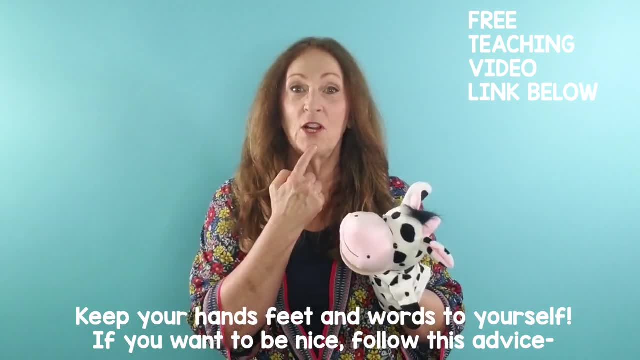 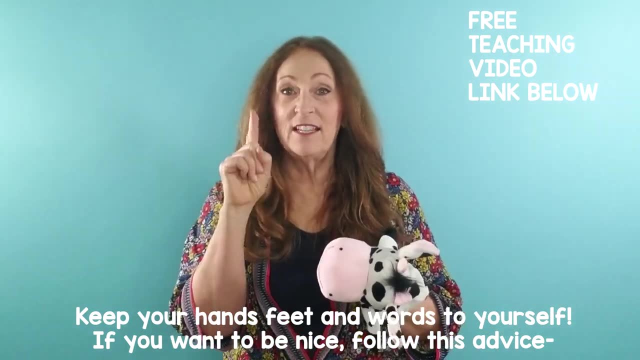 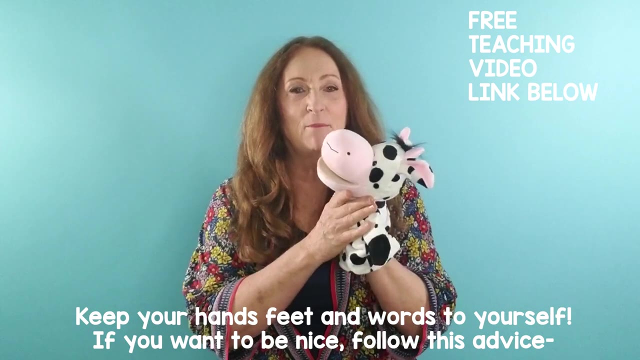 Keep your hands, feet and words to yourself Clap, Clap, And then you can do the action words to yourself. It's a little tricky. If you want to be nice, follow this advice and then keep your hands, feet and words to yourself Clap, clap. So that's just the easy way you can do it. 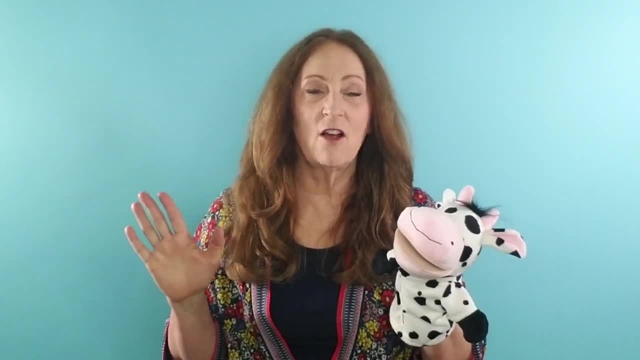 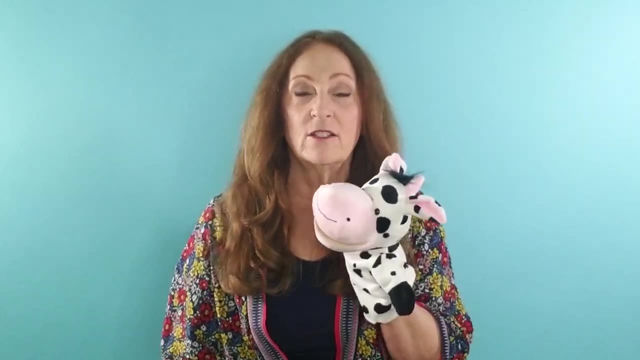 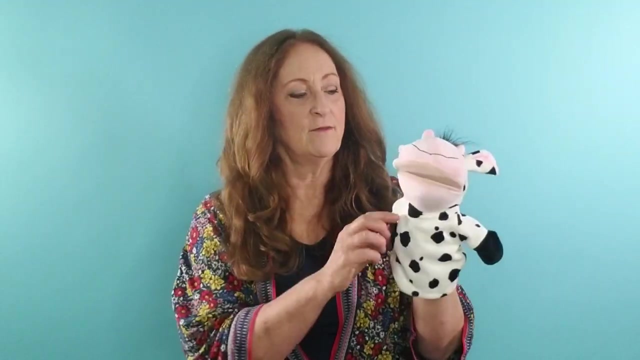 at least to teach the rule. You may not ever sing the song again, but the kids actually do like the song and you can play around with that. And Mrs Cow can also help teach that. You know hands, feet, words to yourself, to yourself. You know make up some funny voices and have fun with it. 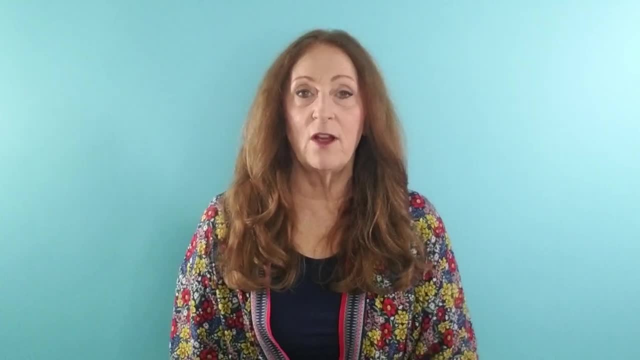 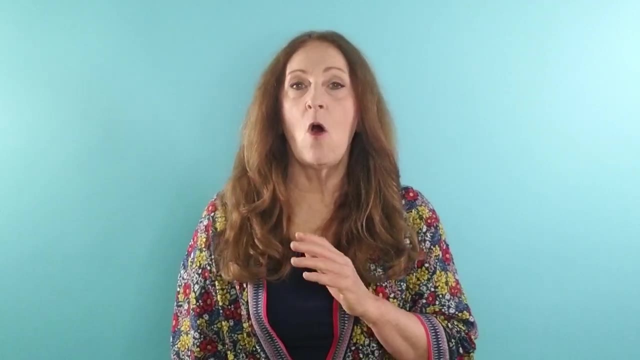 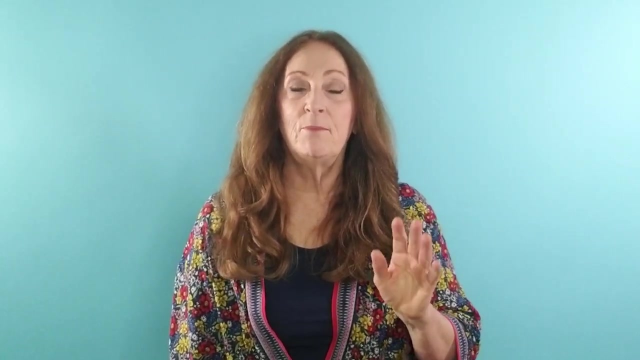 So it's really important to have those procedures and rules and try and weave them into the music activities on the first day, And my personal opinion is to not overload everybody by spending all of your class time on those rules and procedures, but maybe pick the ones that are. 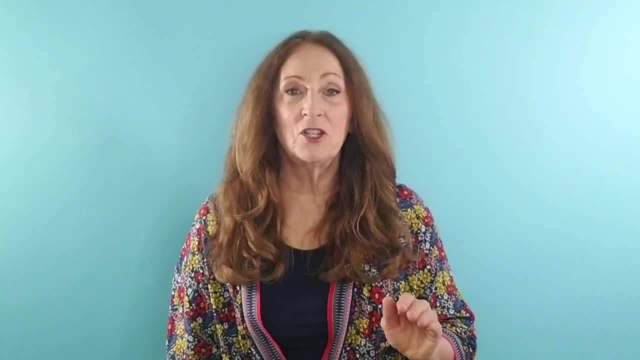 super important for the first day and then make up some funny voices and have fun with it. And if you have any questions, please visit my website at wwwretrainingledcom If you have any, And make sure that you're doing some kind of name game or some kind of connection activity. 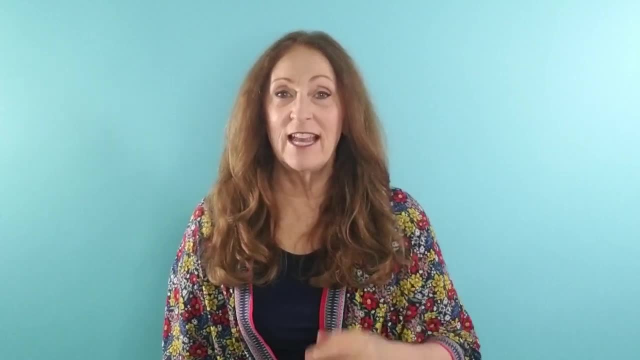 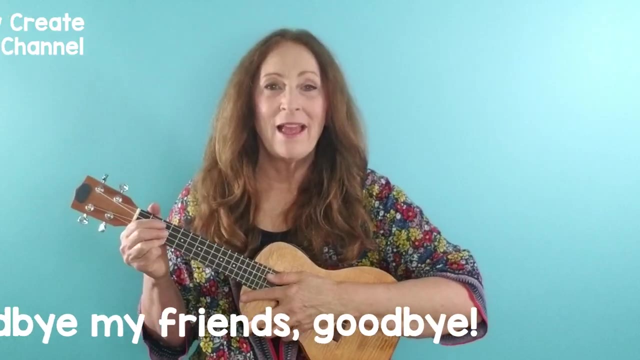 where the students are going to know you and you're going to start to get to know the students, And the hello song that I sang is also a goodbye song, So it's easy to pick up and the goodbye song is actually on the Sing Play. Create YouTube. 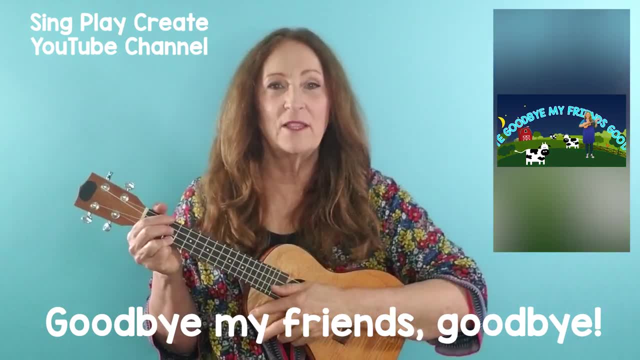 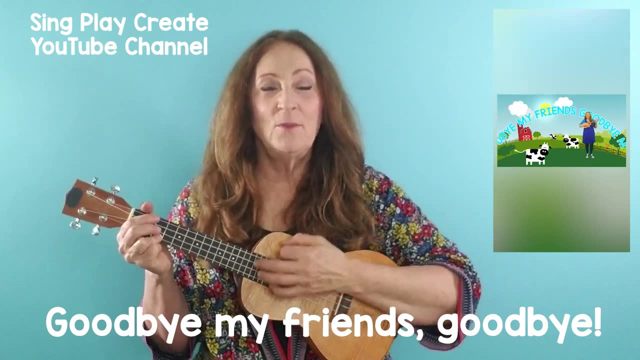 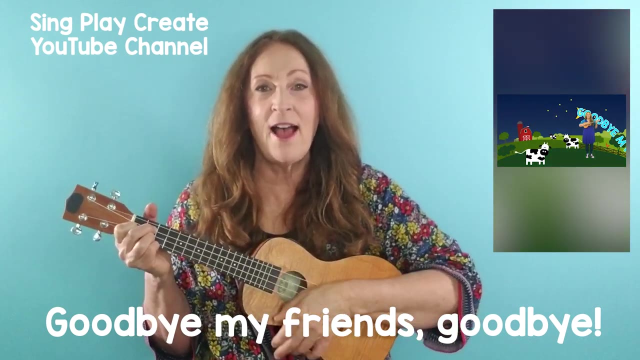 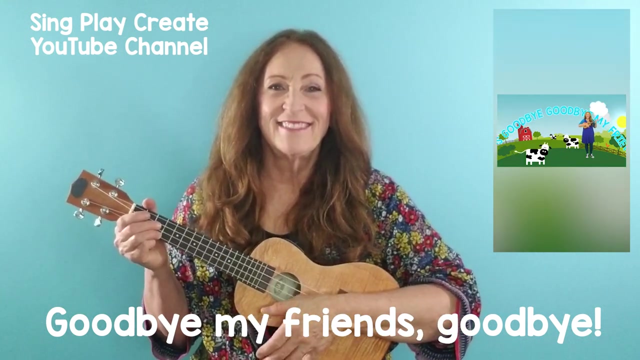 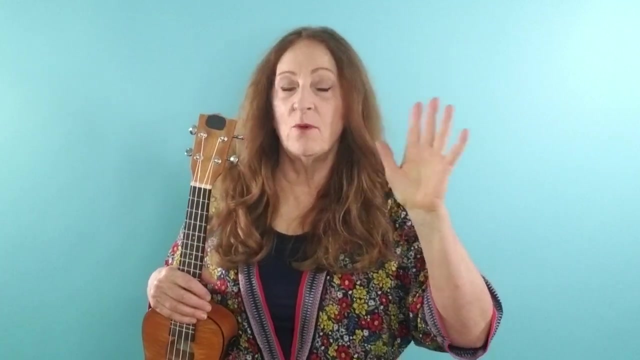 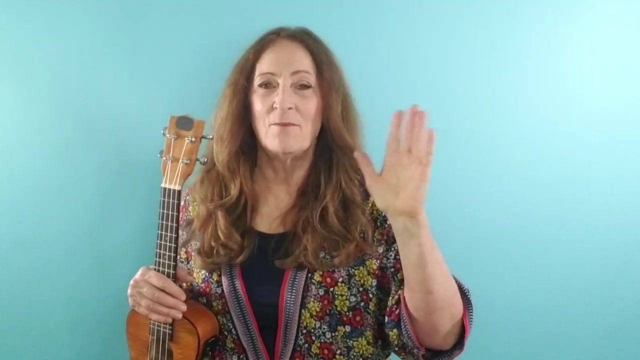 channel and it's really cute and you can sing along with the video. And this is where I teach the kids actually to wave to each other, Because not only are we building connections with the students, But we're helping everybody make connections with each other. 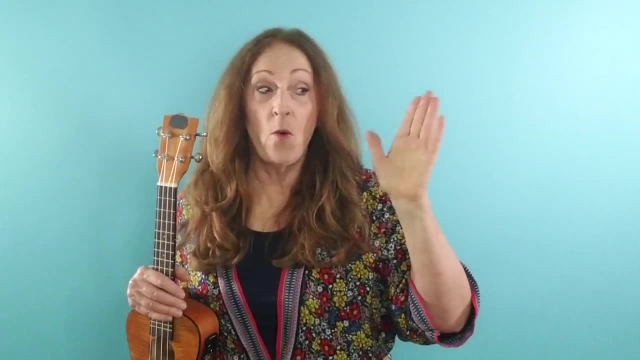 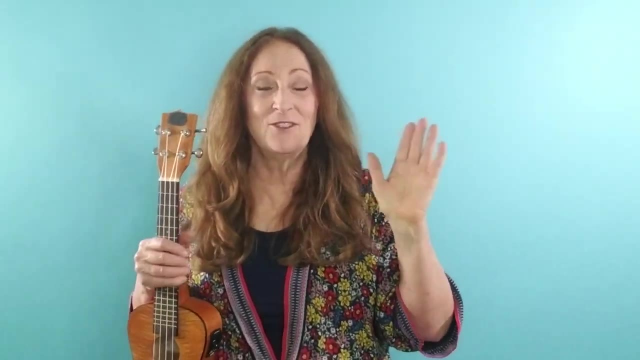 So while I'm singing it the first time, I'll say: okay, everybody, wave to your neighbor and frown, I mean smile. Make sure you smile at your neighbor like I'm so happy to see you and wave goodbye. And you can do that with the hello song too.